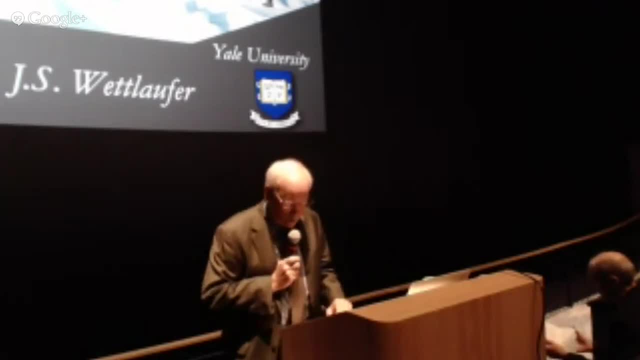 I was thinking of the fifth IPCC report that came out just a week or two ago and has continued to get clearer over the five renditions of that report, stating for the first time that the warming of the climate system is unequivocal: atmosphere and ocean have warmed amounts. 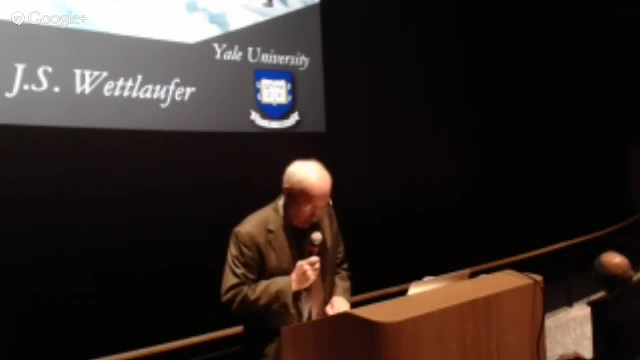 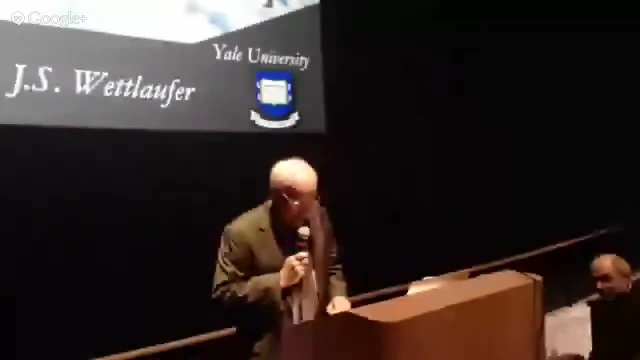 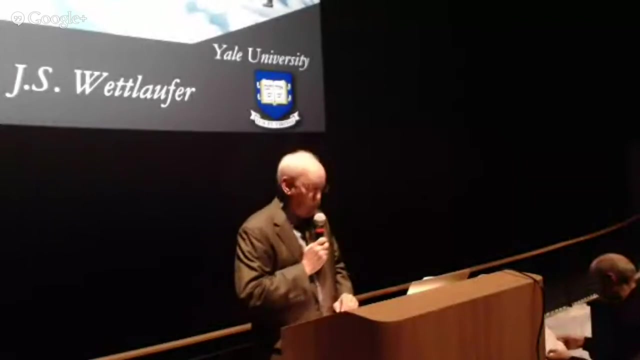 of snow and ice have diminished, sea level has risen. That much is known and sounds elegantly simple. but documenting exactly what has happened in the past and what may happen in the future, and most importantly, why, is much more difficult. It's equally challenging to try to explain what we know and what we don't know to the 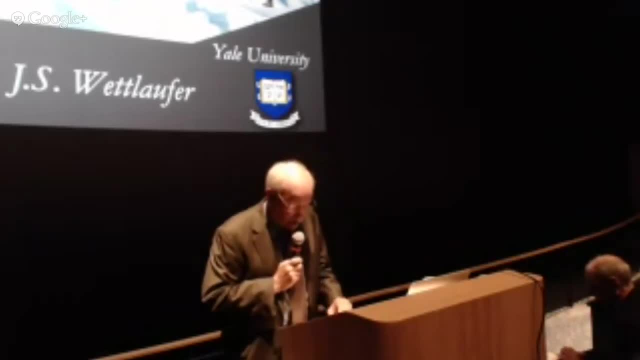 public. That's why the John Carlson Lecture Series is so important and why we are delighted now to collaborate each year. Indeed, we here at the Aquarium share a desire to raise the level of public understanding about climate science and global change. The Aquarium, for example, leads a nationwide collaboration now of 30 aquariums and zoos. 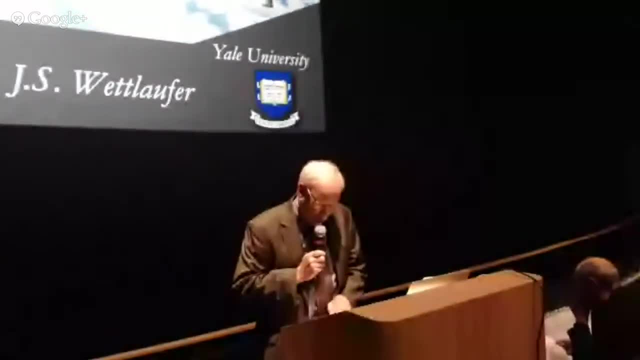 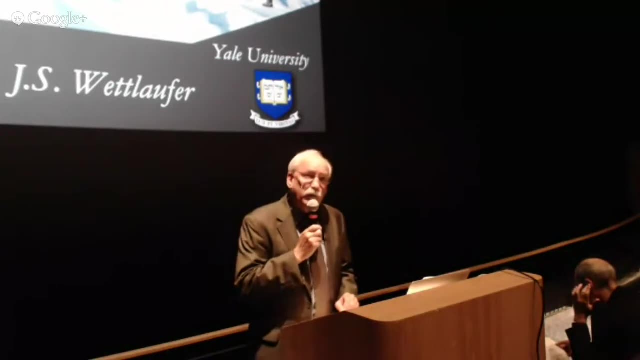 funded by the National Science Foundation and NOAA, working together to figure out how best to educate our visitors, And together we reach almost 30 or 40 million people a year, so it's a great opportunity. That effort, of course, must have a strong scientific foundation under it, which is why 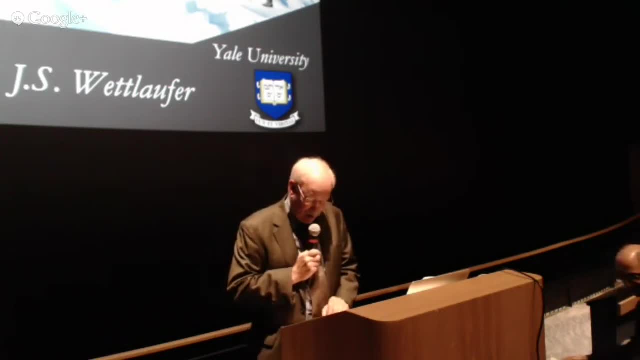 we are so grateful to the work done by the Lorenz Center and again the intention of the John Carlson Lecture Series to bring that work to the broader public. So I hope tonight's presentation will lead all of you to new discussions about global change with your colleagues, your family and friends. 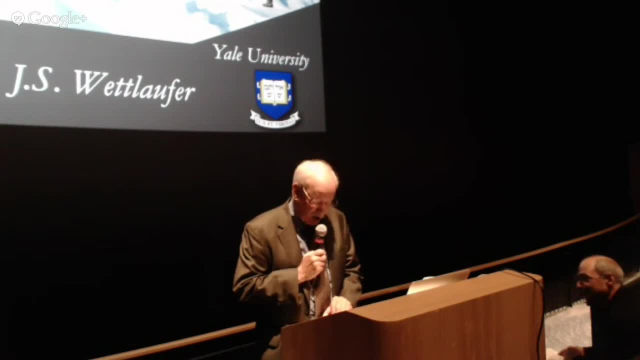 By having such discussions, you too can help to share good information and raise awareness. I'm happy to be joined tonight by Kerry, Emanuel, Cecil and Ida Green, Professor of Atmospheric Science, and Daniel Rothman, Professor of Geophysics, the co-founders of the Lorenz. 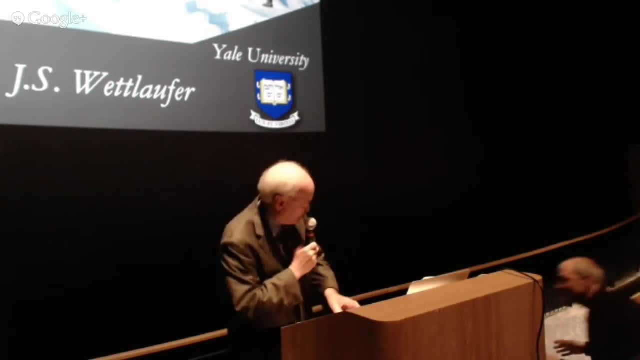 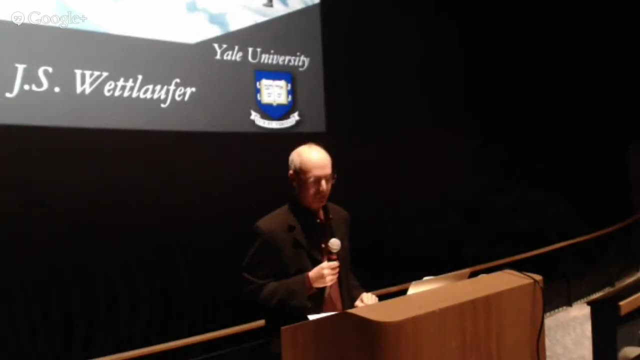 Center and MIT, And I'm going to turn the mic over to Dan. Thank you, Bud. Welcome to the third afternoon. Welcome to the annual John Carlson Lecture. This lecture is made possible by a generous gift from John Carlson, John Carlson's gift. 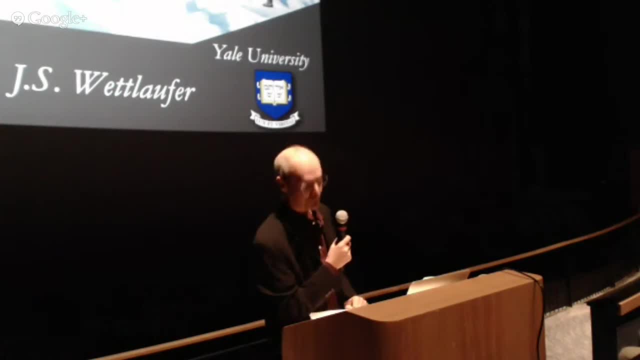 to MIT's Lorenz Center. I'd like to spend just a couple of moments remarking about two wonderful benefits of John Carlson's gift. First, which is quite obvious, I'm sure, to everyone in this room, it provides a way of 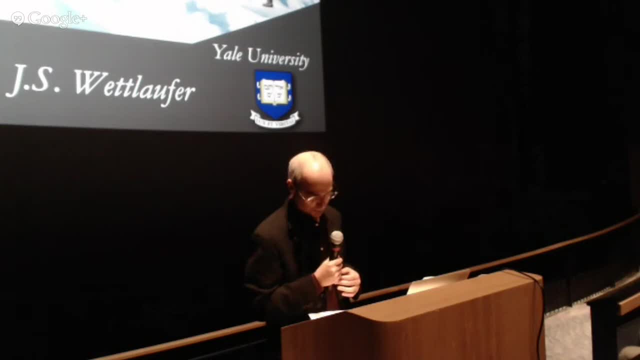 communicating basic climate science to the general public. Thank you In doing so. the Carlson Lecture also honors the legacy of Ed Lorenz. Professor Lorenz is widely known as the father of chaos theory, which he discovered as part of the studies of the predictability of the weather. 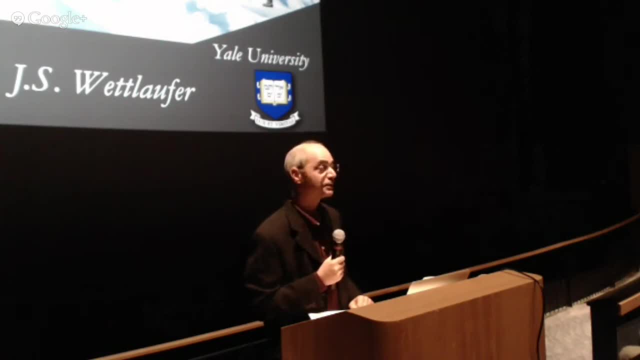 Such curiosity-driven research, performed in the context of an important practical problem, epitomizes the spirit of the Lorenz Center. Tonight's Carlson Lecture Lecturer John Wettlaufer is the first lecture to be held at the Lorenz Center. 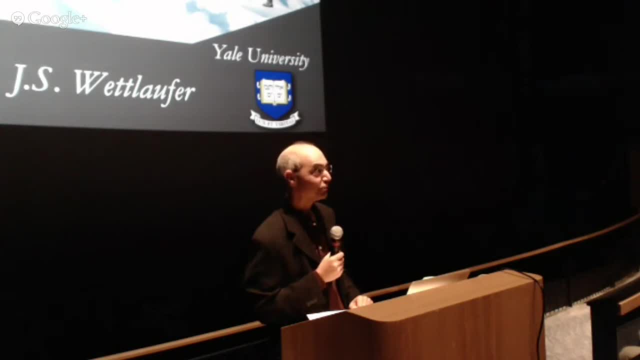 He is Professor of Applicable Mathematics at Oxford and Professor of Geophysics, Physics and Applied Mathematics at Yale. Now, that's a mouthful, but the reality is actually quite simple. John studies the physics of ice. His work is held to explain problems ranging from why ice is slippery to how glaciers 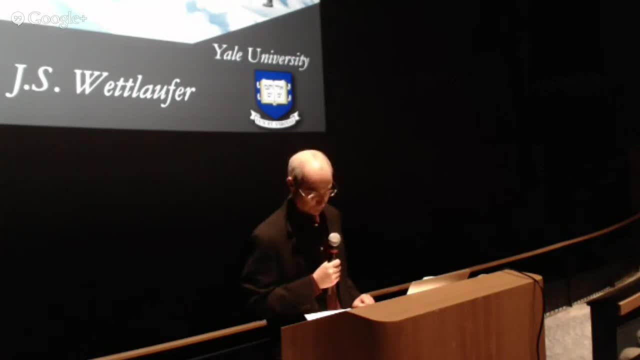 flow. In particular, the implications of his work for improving our understanding of climate has attracted much of his attention and his colleagues. One of the remarkable aspects of John's work is the way he combines fieldwork in the Arctic, laboratory experiments in his own lab, and mathematical theory. 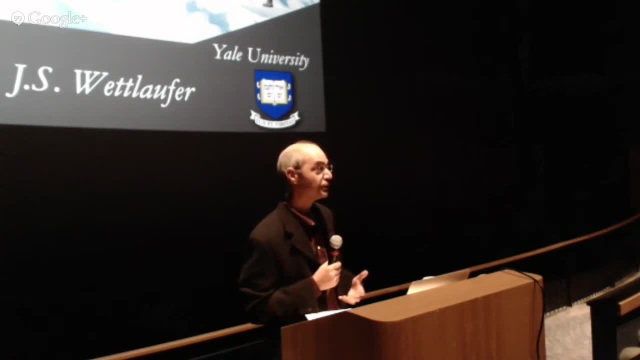 This interplay between theory and observation, so central to basic climate science, is, as you shall soon see, also one of the main and most intriguing features of his work. So, without further ado, let us welcome John Wettlaufer. 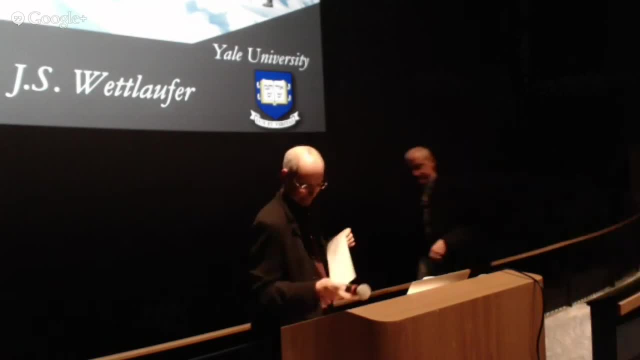 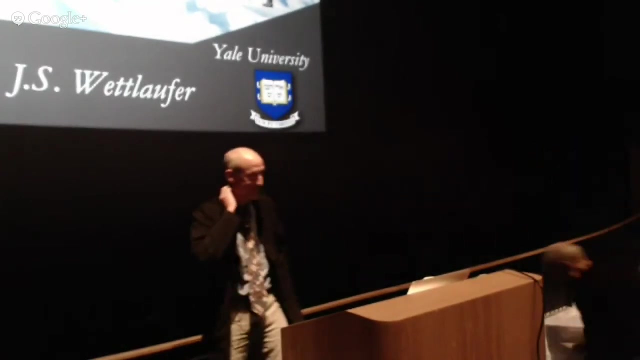 JOHN WETLAUFER, ASSOCIATION TEACHER CONCENTRATING IN INITIATIVE ACTIVITY. Can everyone hear me? No, Yes, No, Yes, Yes, Yes, Yes. Well, thank you very much. I want to thank Kerry and Dan and John Carlson and the Aquarium and MIT for inviting me to. 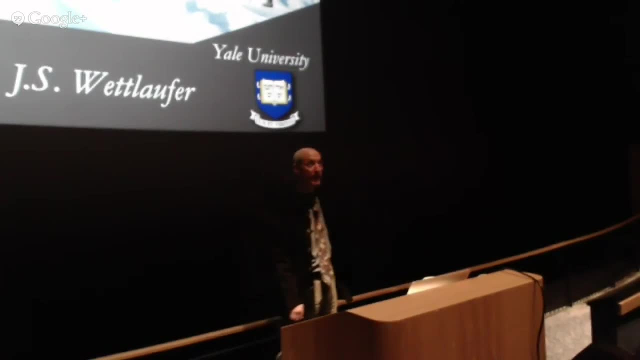 join us here today. I have talked to John twice and he is a professor and professor of science at MIT, inviting me to help celebrate the aspects of the legacy of Ed Lorenz by taking you on a kind of tour of my particular view of what we understand and what we don't understand. 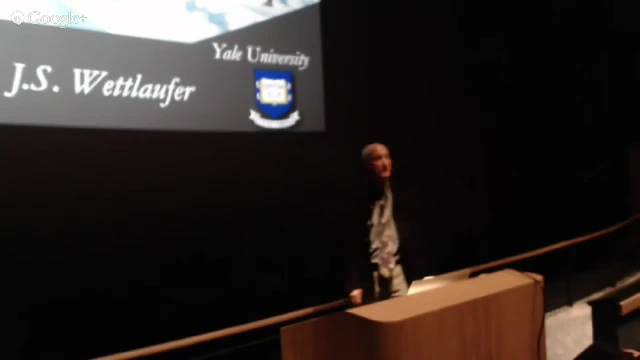 and why and how it sort of fits into the pantheon of physical sciences. Now I don't often get the chance to stand in front of this big screen like this. When we were in Stockholm last year, we used to go to the National History Museum and go. 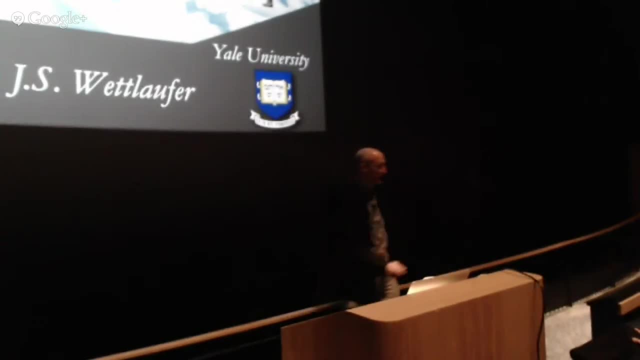 to the IMAX theater all the time, and when my son finds out that I was standing here and didn't come out of the screen, he's going to be sorely disappointed. Okay, And I'm going to have a little bit of a break. 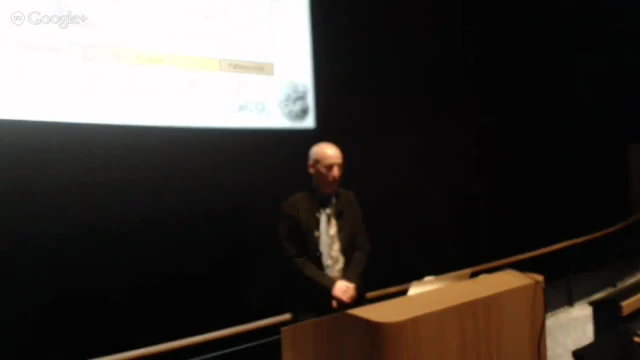 I have trouble sort of seeing where I'm going, but this is a picture of the way in which people who do geochemistry try to understand the fluctuations in our past climate. I'm not going to dwell so much on this, but to say that there are proxies that allow one. 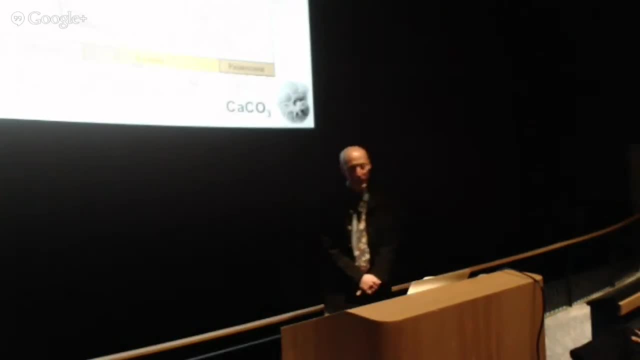 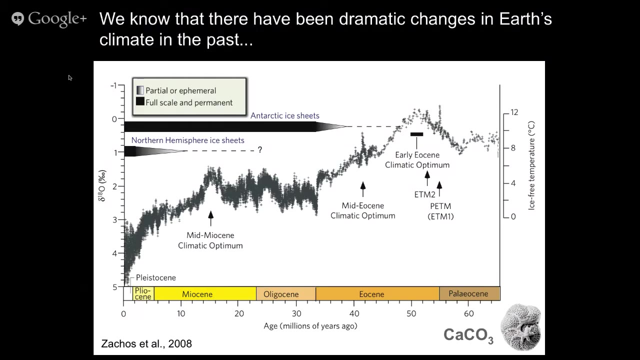 to look at temperatures in the past climate, and this is one of them, showing you over the kinds of timescales that you're not used to, sort of digesting how the temperature has changed. And you can see on the right-hand side there is the temperature and the past, and, as you 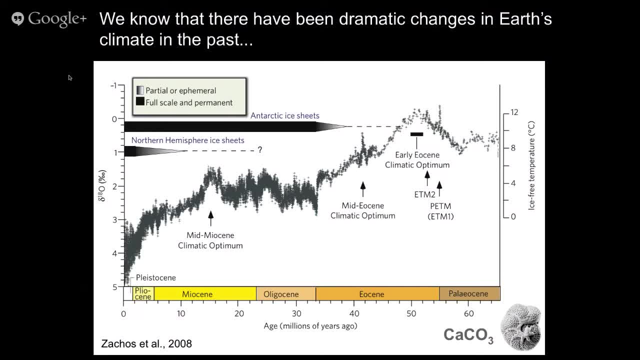 go from that side to this side. you go from then to now and Is there feedback? I think there's. Do you have the other mic? Yeah, Okay, Okay. so you see these wiggles and you see dramatic changes in the past climate record. 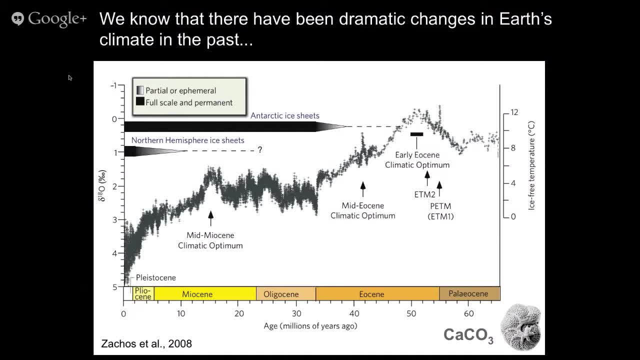 You see that ice in the Southern Hemisphere is a rather new entity on a timescale of 60 million years, and in the Northern Hemisphere it's even more of a recent phenomenon. So it's very interesting to see how climate change has changed over the last few decades. 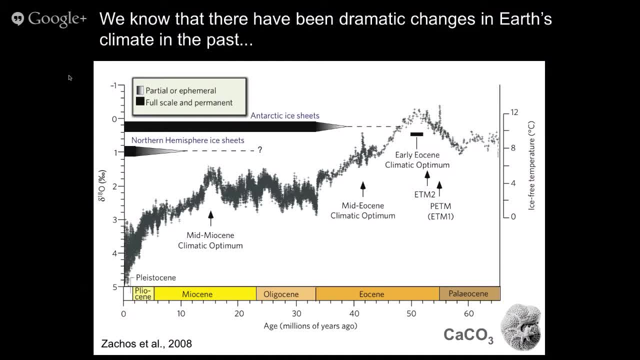 And I think it's interesting to see how climate change has changed over the last few decades. And I think it's interesting to see how climate change has changed over the last few decades. So it's very clear that there have been serious changes in the past and the question 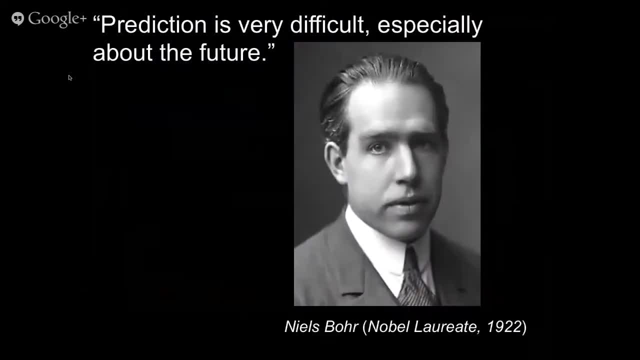 is what's going to happen in the future. So this is a very well-known physicist who is accounted with making this statement. It's certainly true, And the answer is, of course, we're not sure. So the answer is, of course, we're not sure. 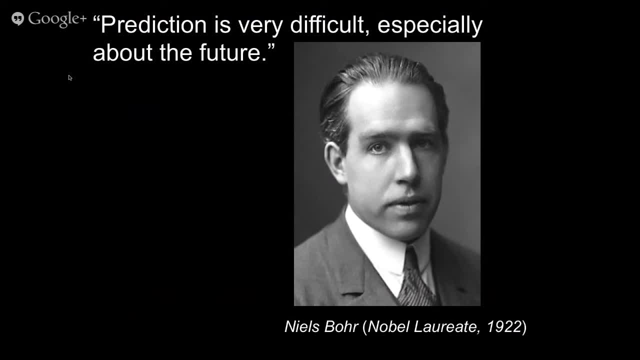 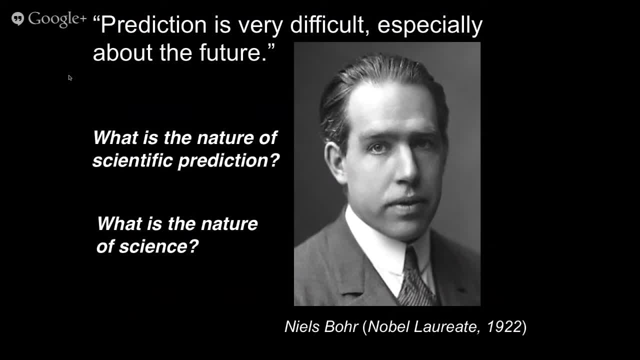 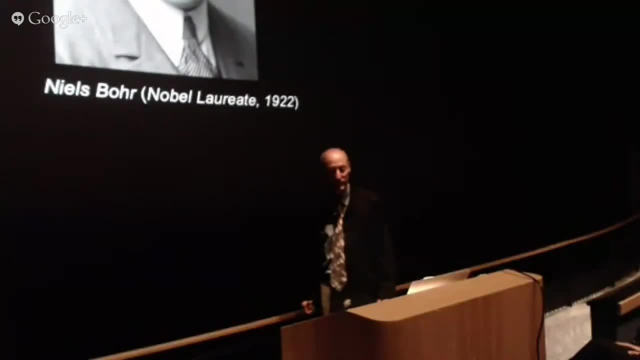 And, in fact, what is the nature of science? So of course, I don't know all of you people. I don't know how many of you decided that you would abandon the nature of science in the past and never think about it again in the future, or whether you have a good idea of the nature of science and or your particular 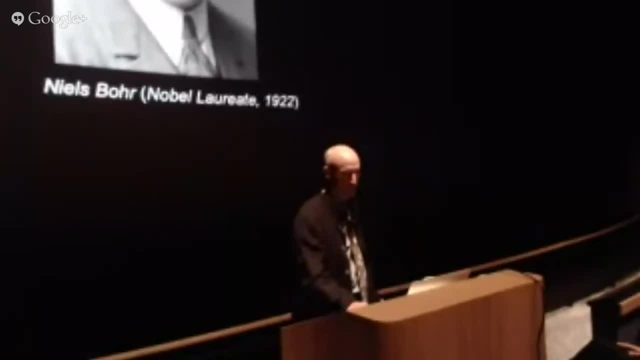 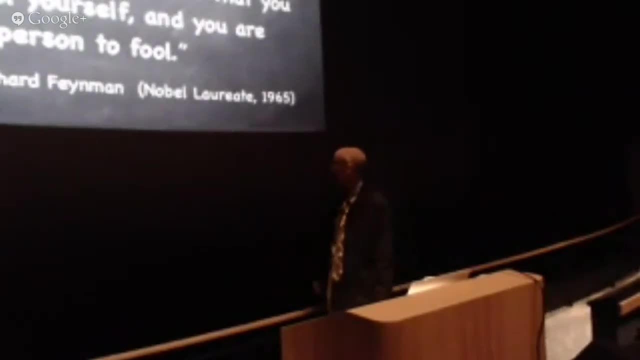 view of what science is. but let's just start with that question, and we'll use one of the great teachers in my field, Dr Feynman, who made this profound statement, which is true: science is a way of trying not to fool yourself, and the first principle is that you must not. 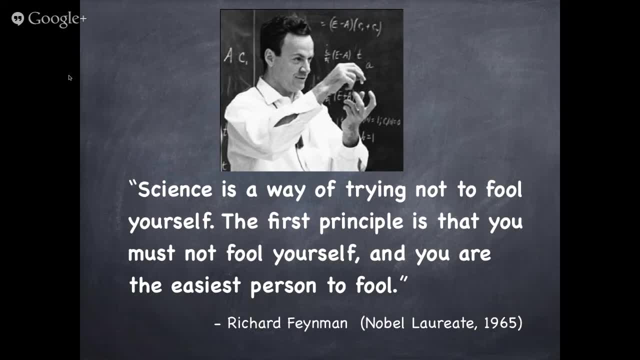 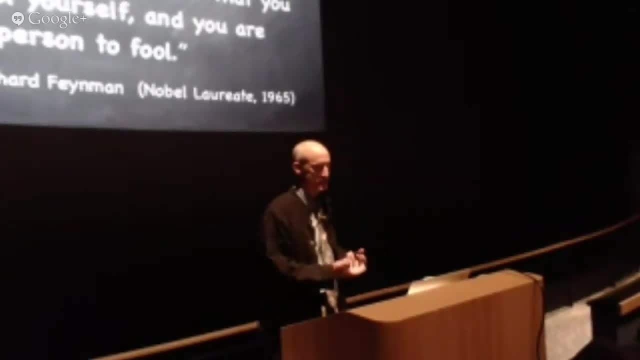 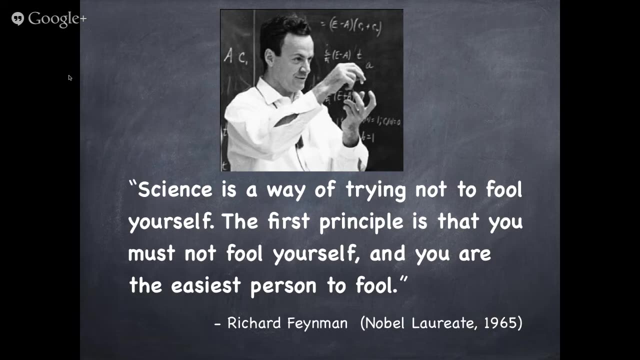 fool yourself, but you're the easiest person to fool, It's true, But it's a deep statement that there are things that just are inviolable, and one of those is that you can't really deceive yourself and the construct of science is really essentially. 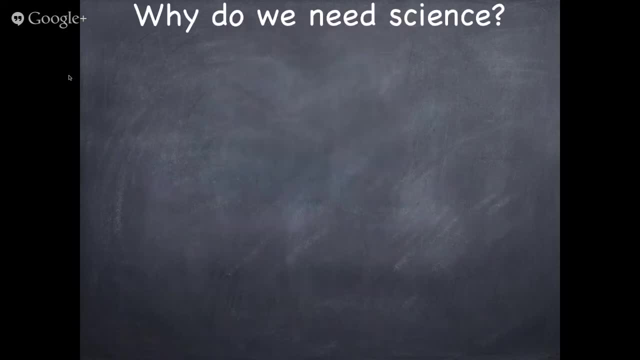 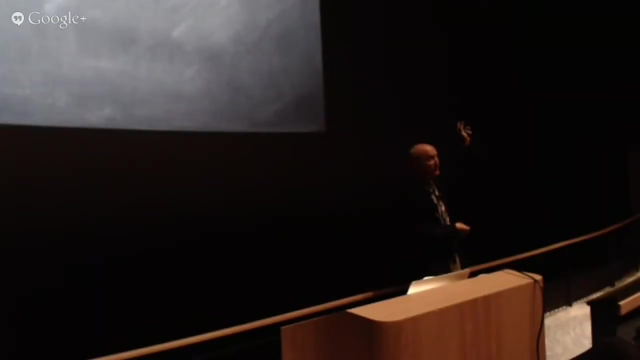 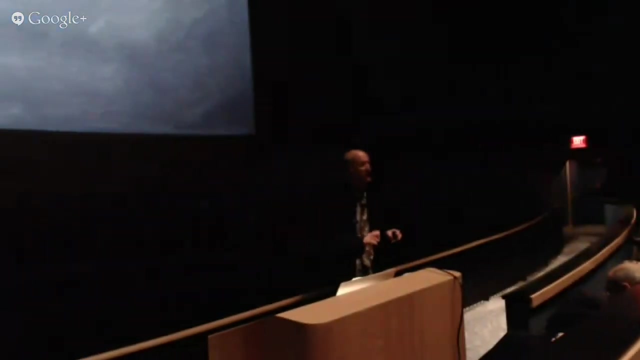 based on this idea, We can ask why we need it, And I'll turn to something that's rather more common for most people. How many people have a cell phone? How many people are extremely annoyed when you don't have any bars? How many people think it's their right to speak on their phone at any time, any place? 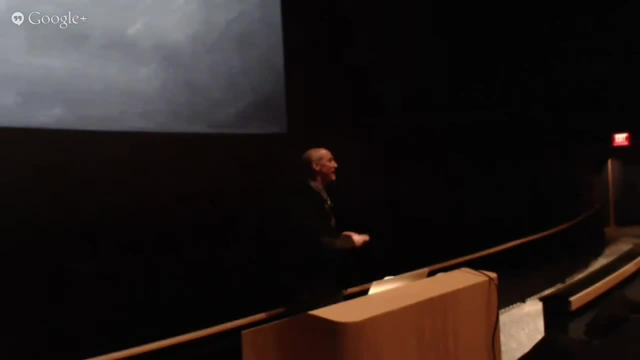 Okay, I'll stop there. Okay, But you demand that the technology works all the time. You drive your car, you use your computer. you're very surprised when it crashes and in fact it's very rare that it really does, given the amount of time you use these things. 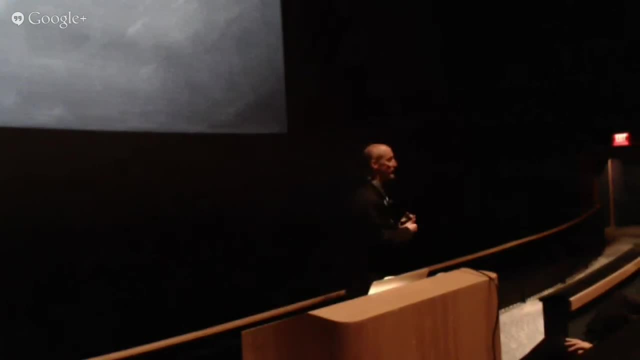 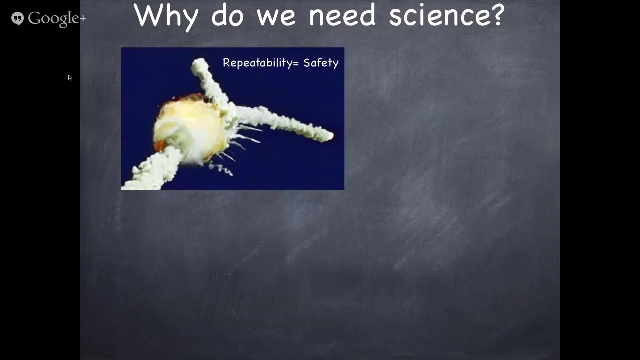 So we often equate technology with science, which is they're obviously related. We need science for repeatability, And repeatability is equal to safety. If you are old enough to remember the Challenger disaster, I remember exactly where I was. 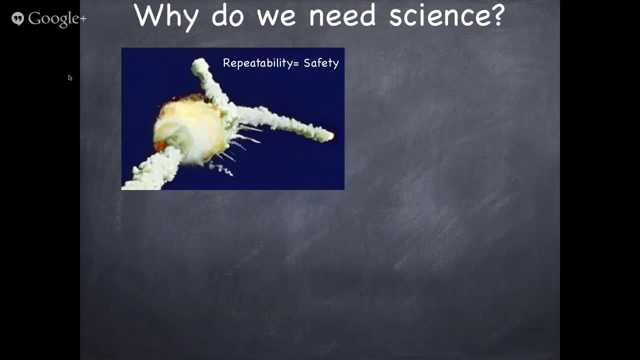 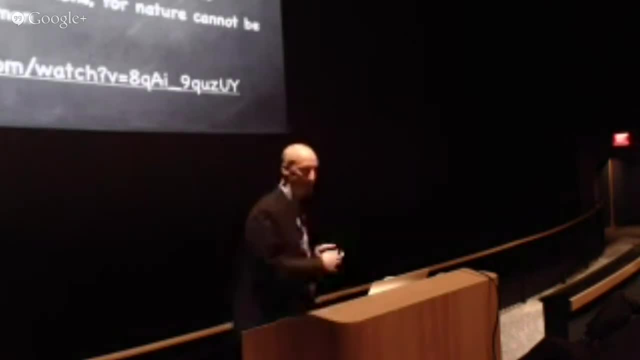 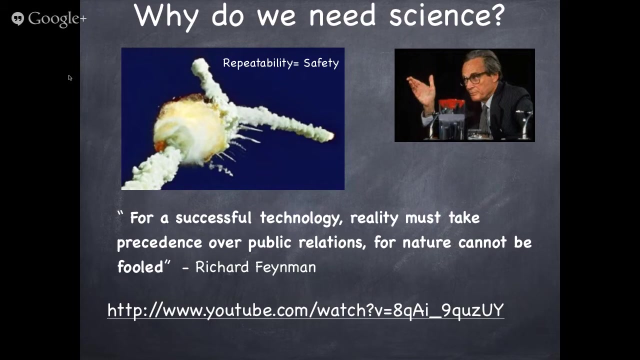 when it happened. the question of what happened there has to do with repeatability and safety and a scientific principle- and I refer again to Feynman who says: a successful technology requires that reality must take precedence- And the answer is that reality must take precedence over public relations, because nature cannot. 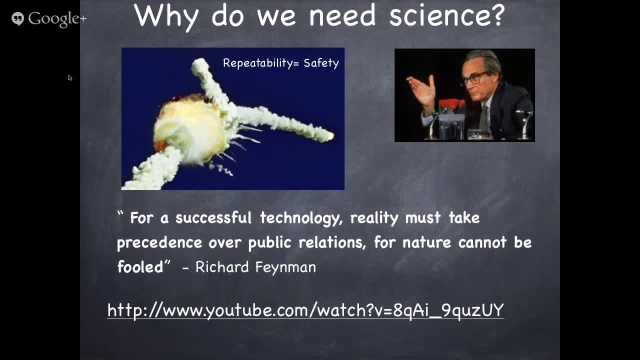 be fooled, And he was asked to be involved in this investigation and his questions were focused on scientific issues. What could have gone wrong? And, as you may know that the O-rings for the solid rocket boosters did not have a high-enough- 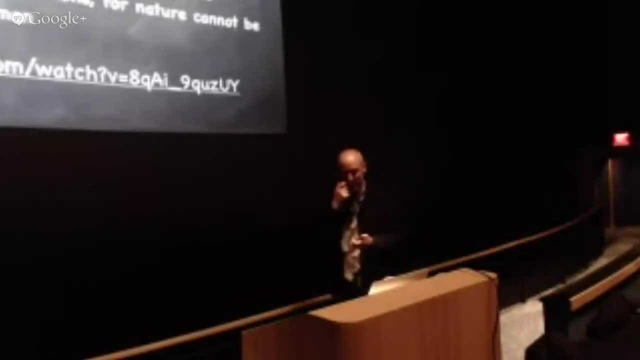 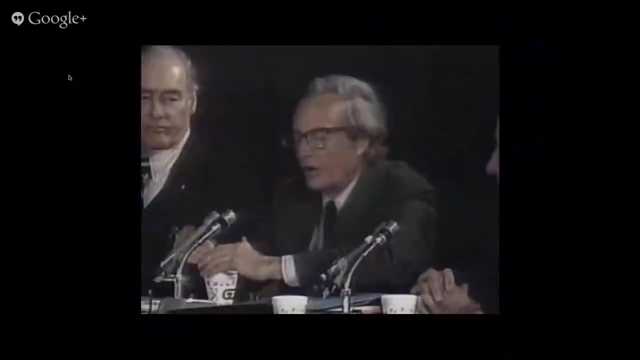 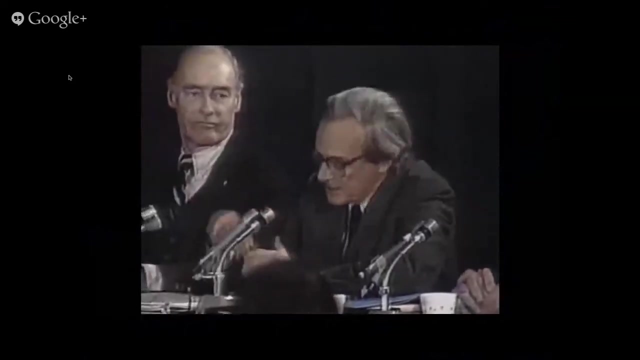 thermal expansion coefficient. They didn't have a high-enough thermal expansion coefficient And that was the origin of the problem. and he sort of demonstrated it here when he did this experiment. And I put a nice one and I discovered that when you put some pressure on it for a while, 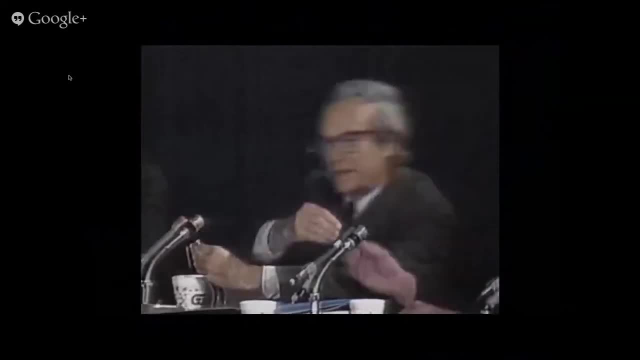 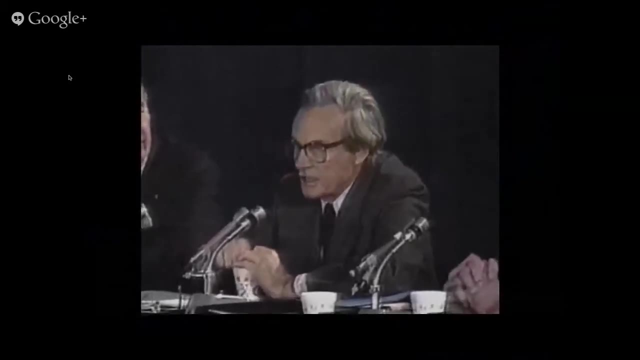 and then undo it, it maintains it doesn't stretch back. it stays the same dimension, In other words, for a few seconds at least, or more seconds. there's no resilience. So if you put some pressure on it and then undo it, it doesn't stretch back. and then 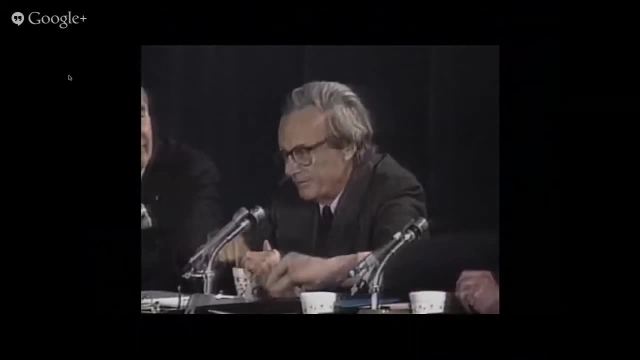 it stays the same dimension. So it's not a real problem. It's a real problem And that's why I think that the O-rings in this particular material, when it's at a temperature of 32 degrees, I believe that has some significance for our problem. 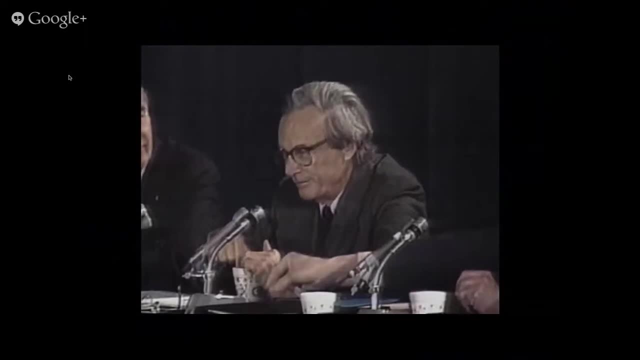 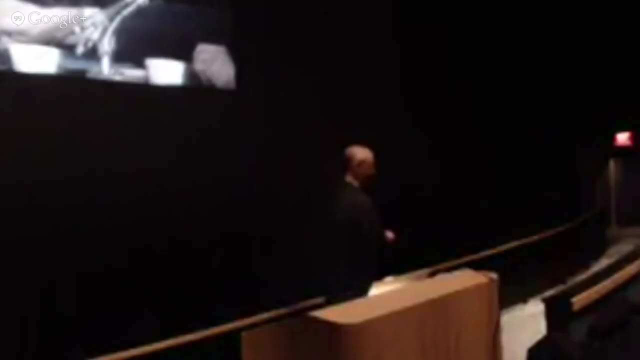 Well, I mean the echo wasn't really part of the original video, but you see what he did right? I mean he tested a very simple scientific principle and saw that there was no resilience in the O-ring. So one might generalize this. 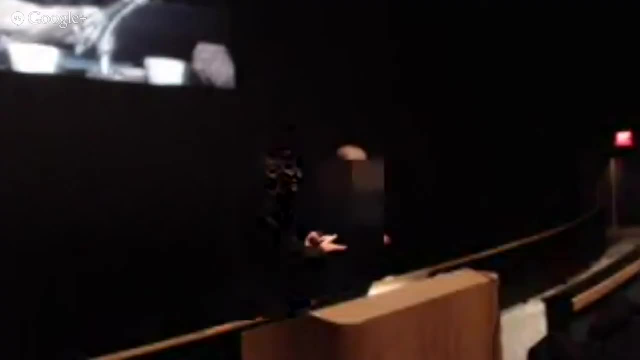 The O-rings are made of a very simple material. They're made of a very simple material. They're made of a very simple material And they're made of a very simple material, And so we generalize this statement he made to. you know our problem. 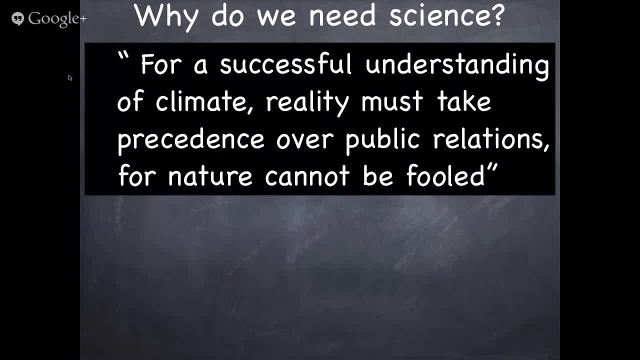 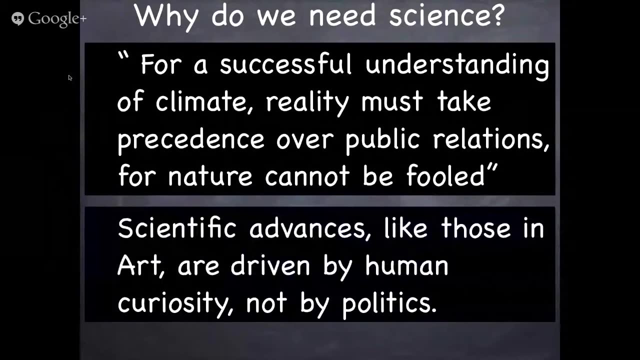 A successful understanding of climate. reality must take precedence over- So it really is true, when we think about it, the lens- that real scientific advances are analogous to those in art. They're driven by human curiosity first, And not by any other way that we can put it. 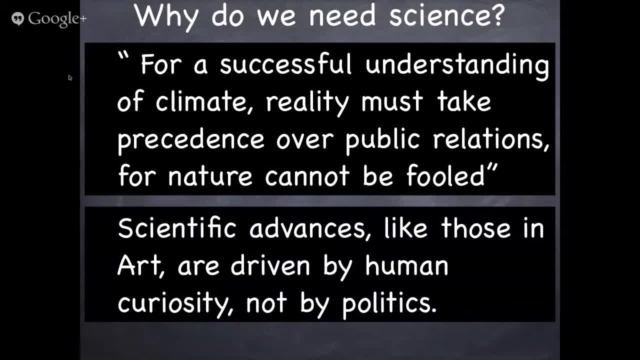 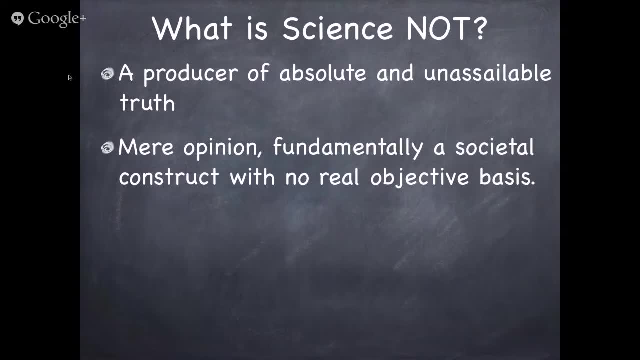 Yes, anything having to do with politics. People who are working hard on science are mostly interested in trying to figure out what's going on. What is science not? It's not a producer of absolute and unstable truth. It's not mere opinion. fundamentally, 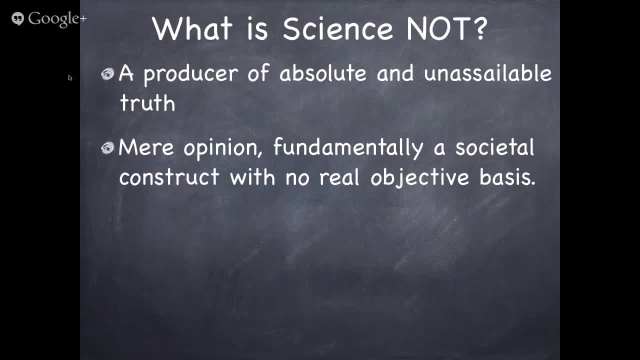 a societal construct with no real objective basis. It's not that either. It's a tortuous process. There are recipes, even though you may have been led to believe that in high school, one makes incremental tests and tries to make progress towards repeatability. 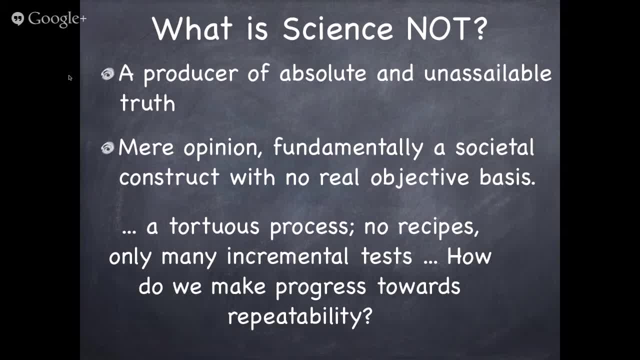 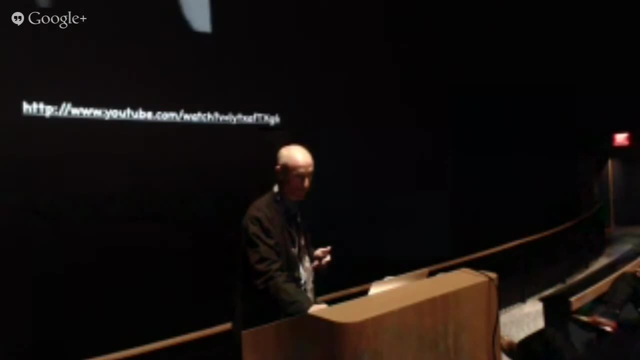 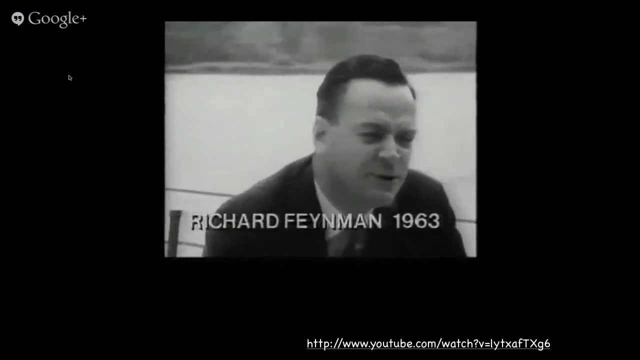 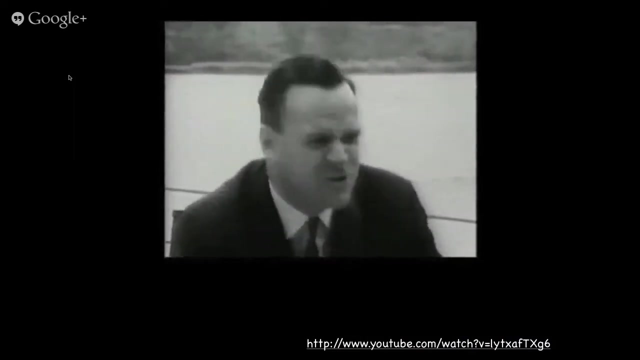 Now, anyone who's tried to figure out something knows exactly what this means. It's a process, A difficult process, and it's best described by Feynman: We put the sticks together to reach the banana and we can't quite make it the idea. 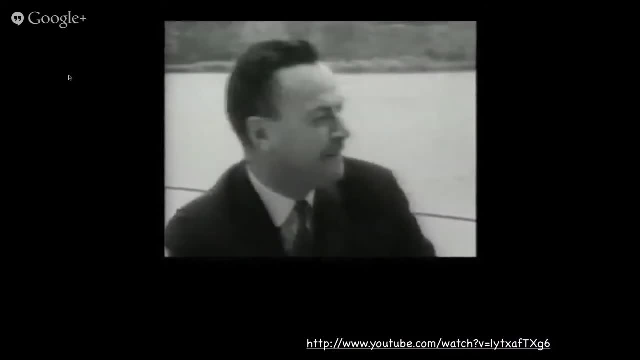 And I get that feeling all the time that I'm an ape trying to put the sticks together, So I always feel the same way. Once in a while, though, every piece of banana, the sticks go together on me and I reach the banana. 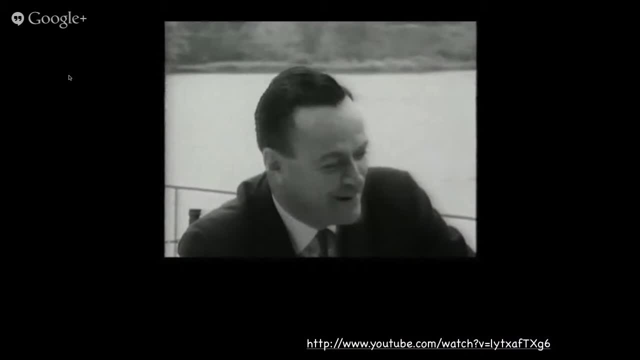 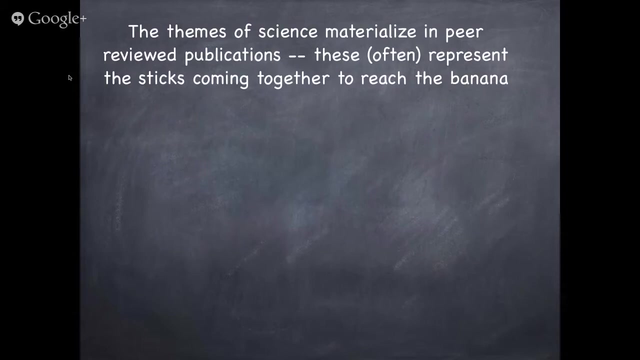 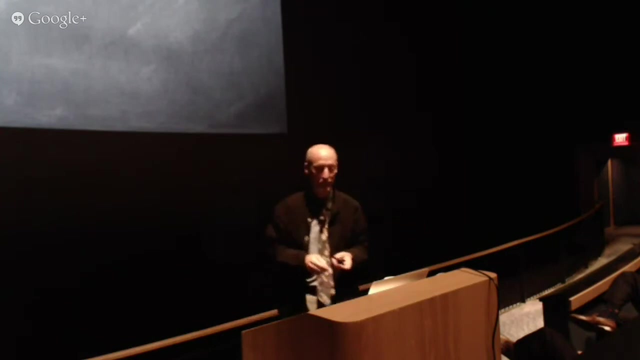 Any one who knows Feynman would be happy to have some of the sticks that he uses. So the idea of when you get the two sticks together is really most represented in scientific papers. All the confusion is usually not published. usually What I tell my group is that if they go home less confused 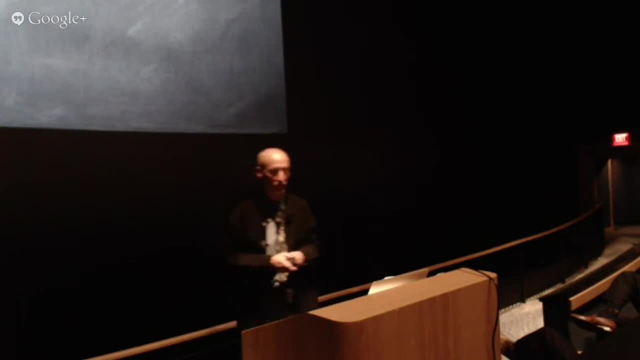 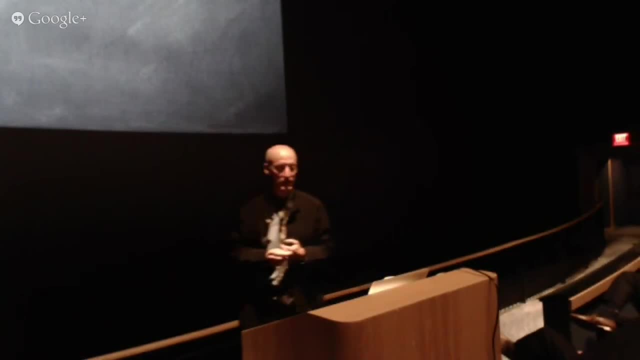 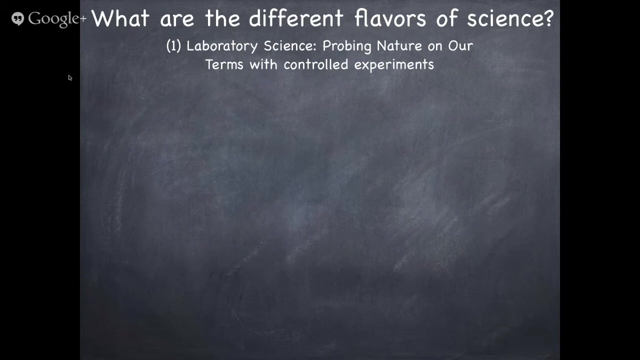 And how do they bear on the particular issues of climate science? Well, there are really two flavors. One is what I call laboratory science, in which we probe nature on our terms using controlled experiments. So just to give you an example, here's: 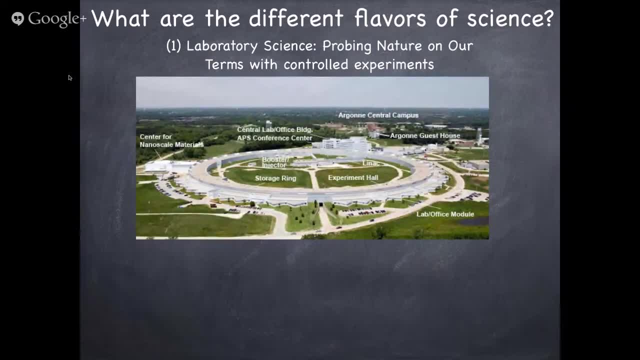 a picture of the advanced photon source at Argonne. You can see there's this big ring And those things down at the bottom are cars, And then this produces synchrotron radiation And you can use that to probe the nature of matter. 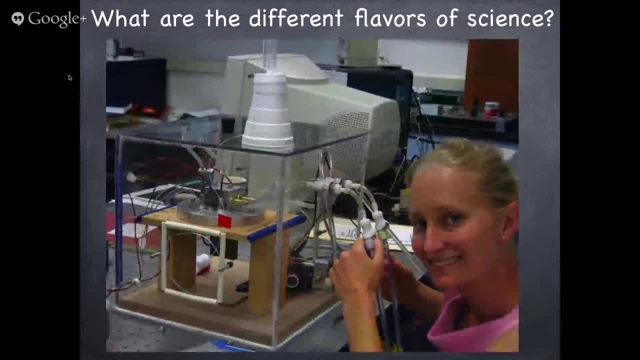 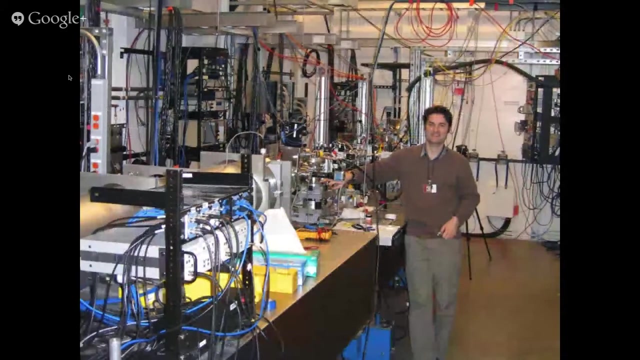 on your terms. This is Melissa Spaneth, who, I can tell you, definitely probes nature on her terms. She built this thing, which is inside this box, And then Steven Pepin installed it right there where his hand is And his sort of simple-looking apparatus there. 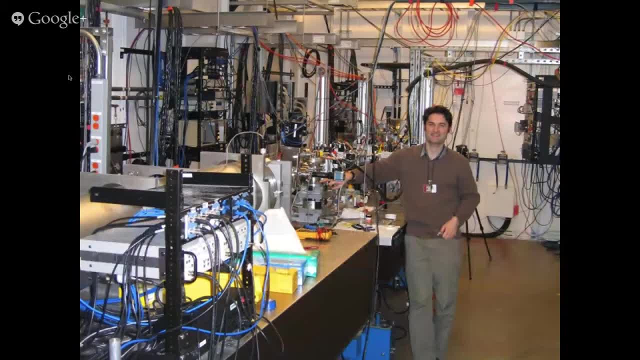 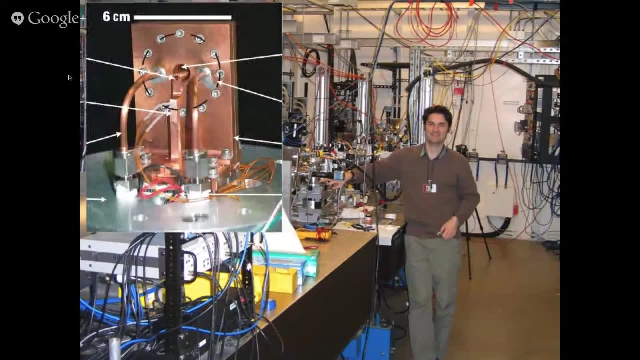 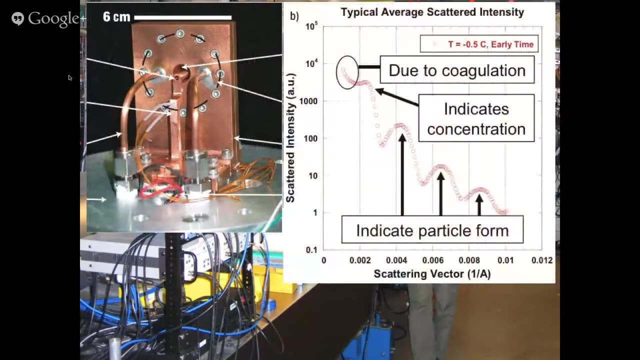 through which some high-energy x-rays are brought in that hole, in this little object there. And my point only is to say that one takes data which this data doesn't really particularly matter, except for if you look at the horizontal axis which is the scattering vector, the units. 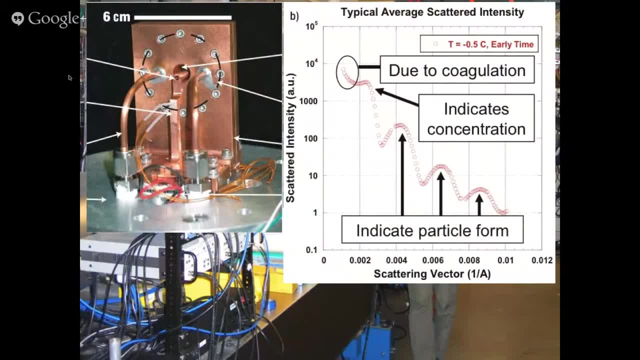 are one over angstroms, So one ten-thousandth of the diameter of your hair. So one can go and probe nature on their own terms, And that's the style of science which you may be familiar with. But it's rather different than the sorts. 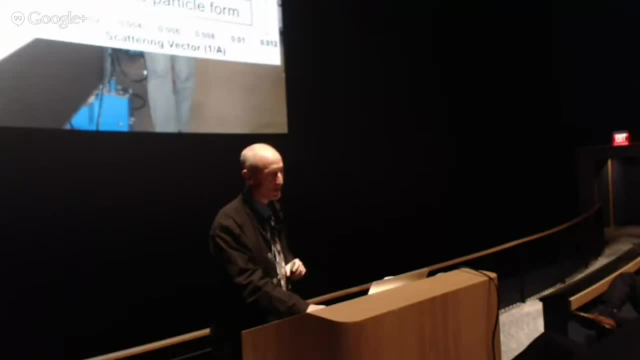 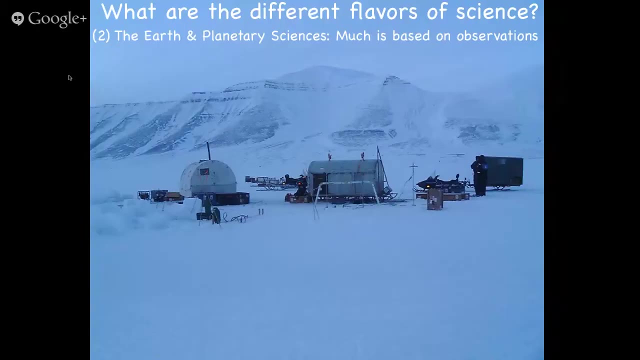 of things one might do in many areas of climate science. The other flavor is based on observation, So one can go and probe nature on their own terms, rather than experiments, if you will, And in that case one probes nature on its own terms. 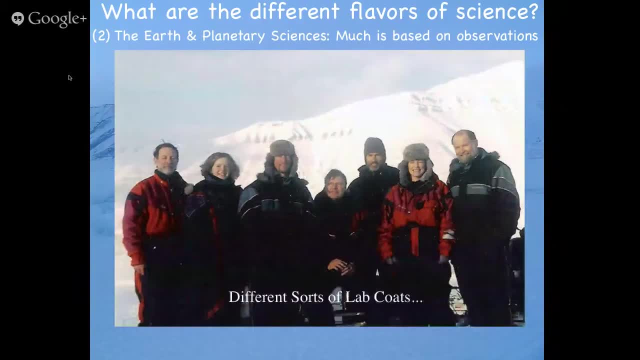 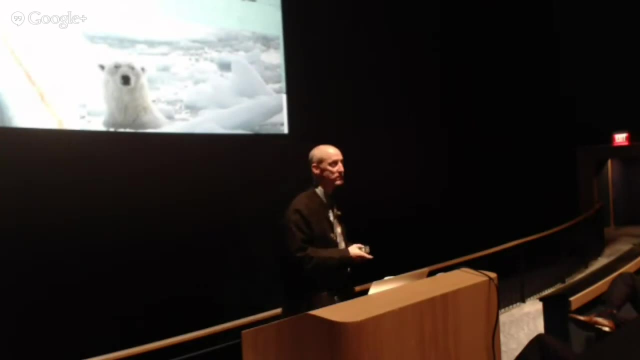 So we have sort of different lab coats. The working day is constrained by various things. I won't ask you who's happy if it's best. The practical consideration is different, rather more than those that one encounters in a laboratory environment. 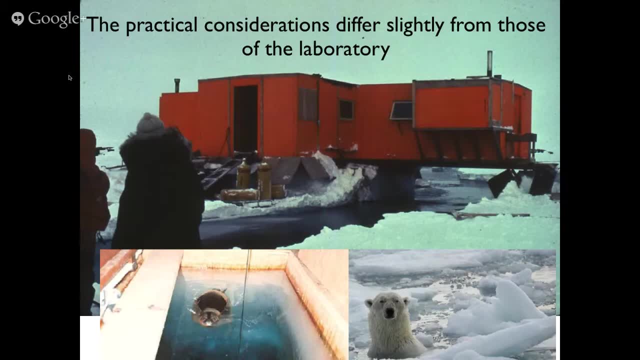 And so you can imagine that people, when they have gone for some period of time under these conditions and have made observations, that they're pretty serious about every data point, because it's sort of hard-won material. But then you have some observations of nature. 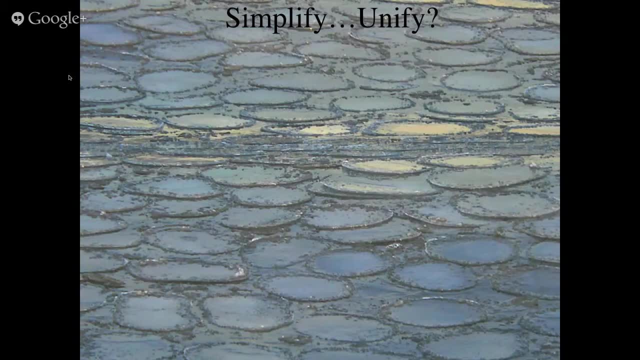 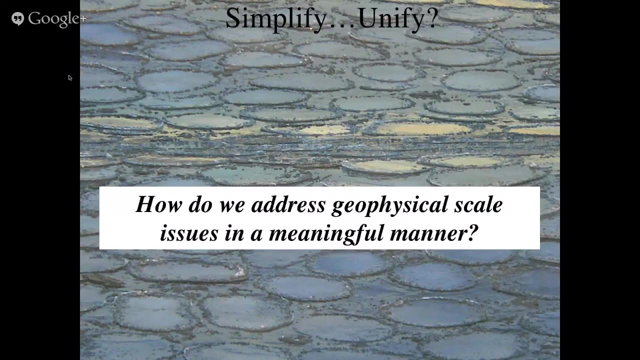 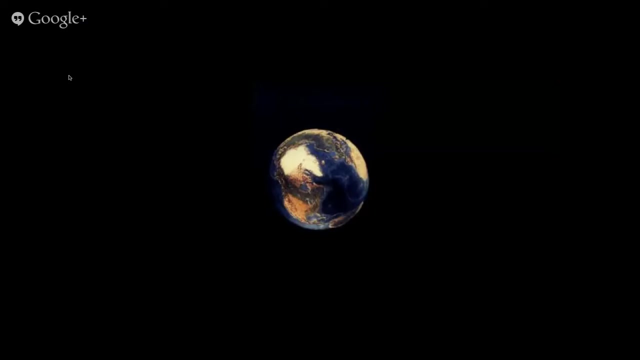 on its terms. and the question is: how do you simplify or unify a complicated system? How is it that one addresses geophysical scale issues in a meaningful manner with local observations? This is a major challenge in this area. OK, so now let's start to take a view. 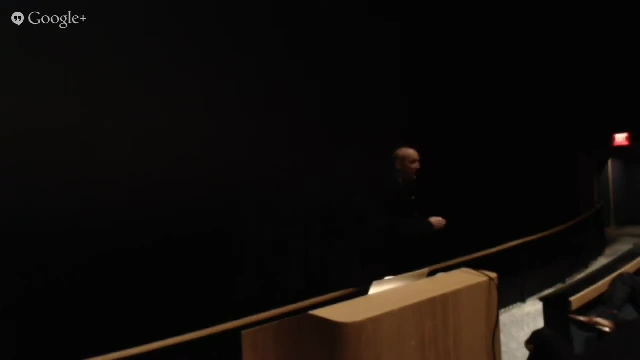 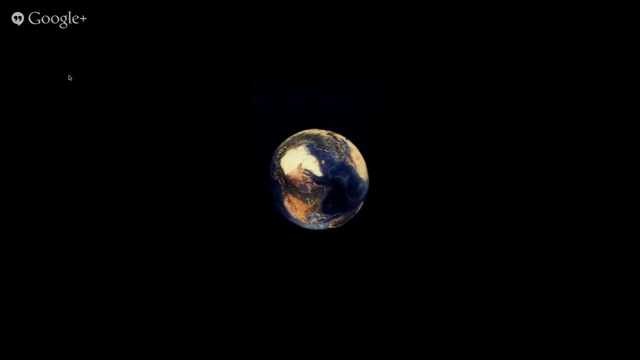 from the north And you may have recognized this object. It's an artist's rendition of the globe, clearly a North American artist, in about June, And so you recognize there's Greenland here, and then this is hard to see because this doesn't really show. 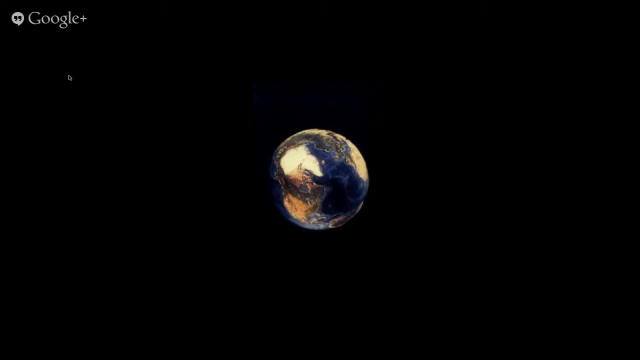 But you see the white cap at the top is the Arctic Ocean And every year the Arctic Ocean freezes and a thin veneer, a relatively thin veneer, persists perennially. It's about 2 and 1⁄2 meters of ice. 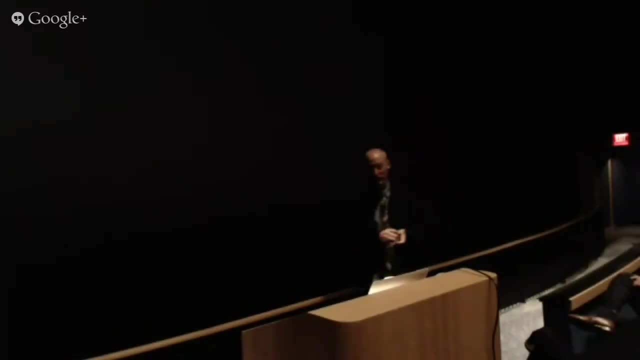 And it grows and decays, and grows and decays, and grows and decays. We'll look at that in a moment. Its importance is multi. It folds When it grows. it rejects salt into the ocean and drives circulations that couple to the global ocean. 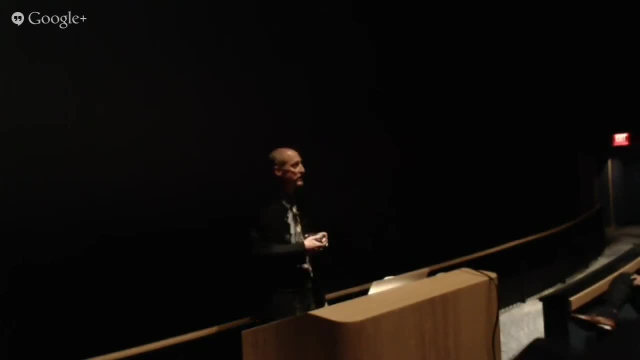 When it expands an area, it increases the albedo of the surface of the planet. The albedo is the reflectivity of radiation, And so white things have a much higher albedo when they're visible than new dark things, And so it's commonly said that the Arctic 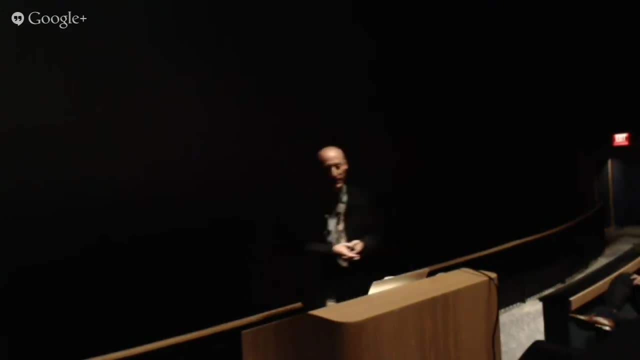 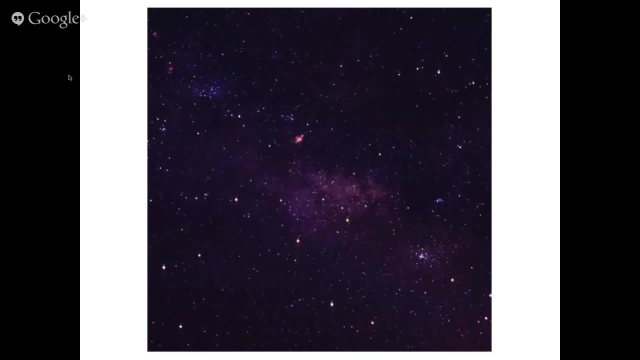 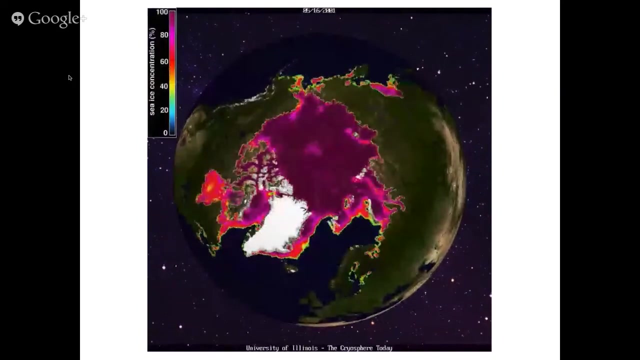 is a bellwether for Earth's climate system. Let's start to parse out why that's actually discussed. Now I'm going to show you a movie here, sped up over six years, And so the color there is. This is looked at from satellite. 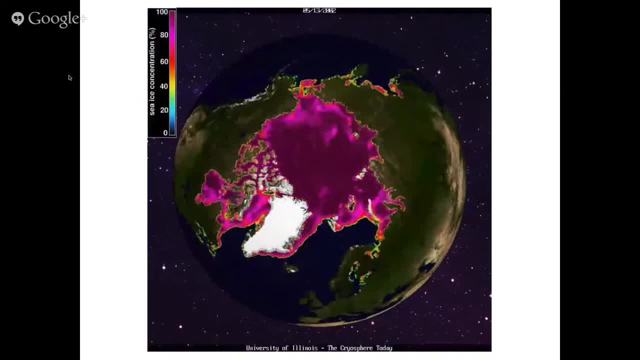 It's the microwave emission of the surface of the Arctic, But the color is the ice. You can see it waxing and waning. That's the ocean freezing And that ice that grows is then ablating every summer, And as far as we are aware, 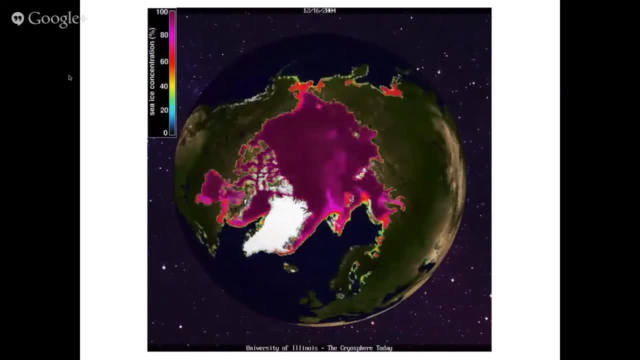 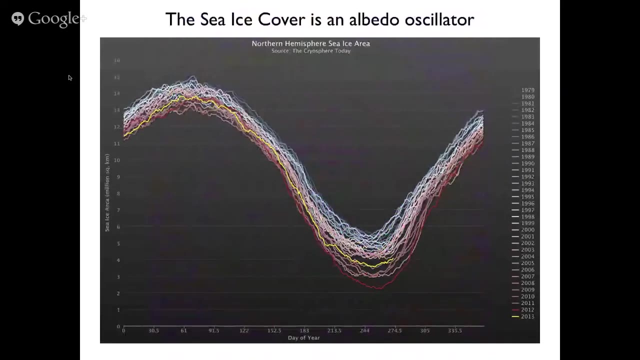 this has been going on for at least several million years. So it's cold, It grows. It's warm in summer It melts back, And from the satellite era, from 1979 until now, this is the oscillation- It grows. 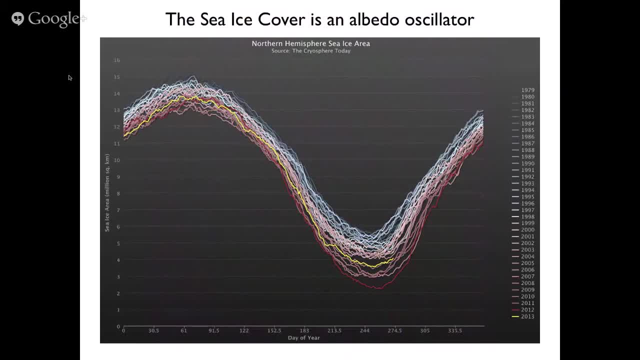 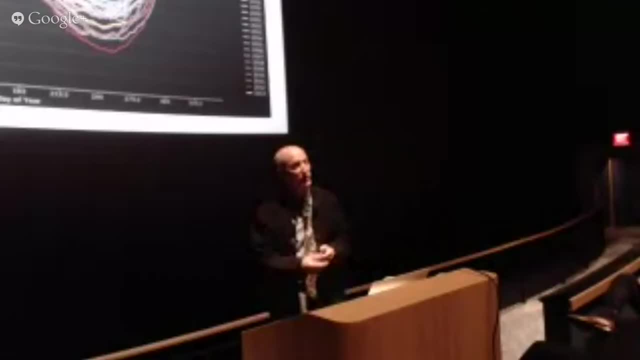 It decays, It grows, It decays, It grows, It decays, And so I refer to it as an albedo oscillator: As the area of white stuff increases, then the area of reflectivity increases, And as it draws back, 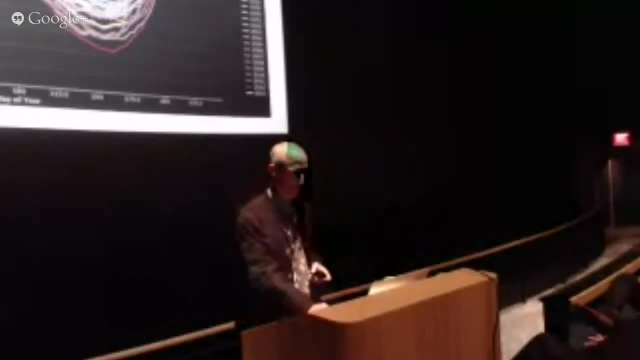 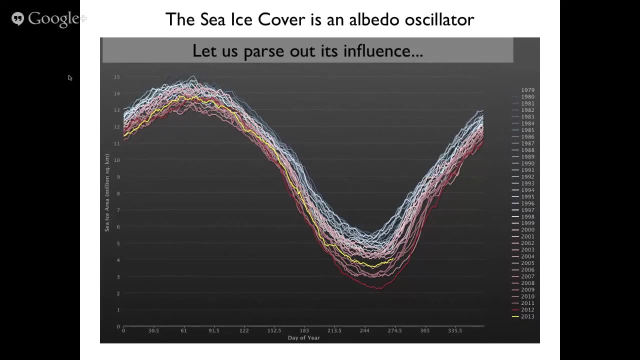 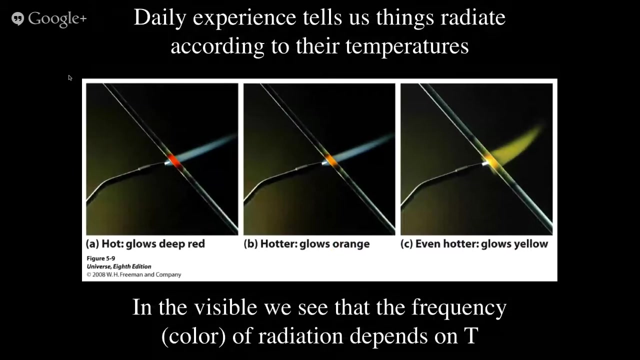 the opposite occurs. So now let's parse out what this really means by a simple argument which appeals to your common experience. So you're familiar with not touching the burner, especially those of you who are children. Don't touch that And it's red hot. 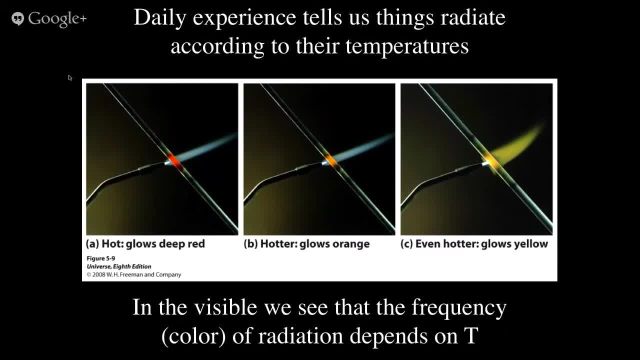 So as you heat up something, it radiates at a different color or frequency. So it goes from red hot up to white hot And you see that the visible emission of the material as it's heated. Now there's other parts of the spectrum. 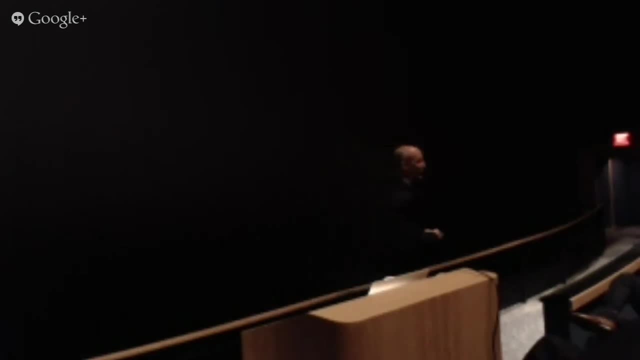 the electromagnetic spectrum that of course, you don't see. You don't see the microwaves that are cooking your food. You need a special way to look at the microwaves. Lately there have been energy audits. Does anyone have an energy audit of their house? 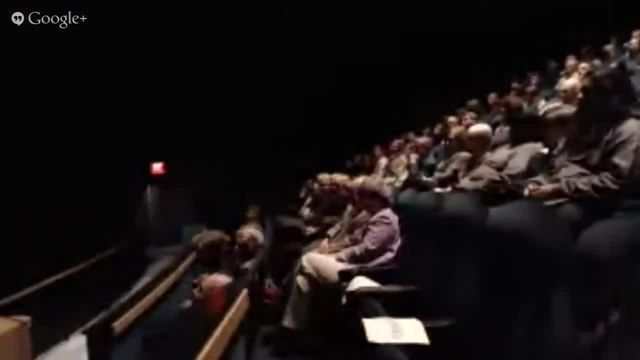 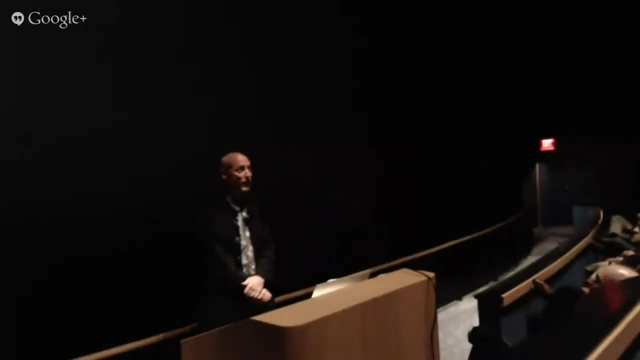 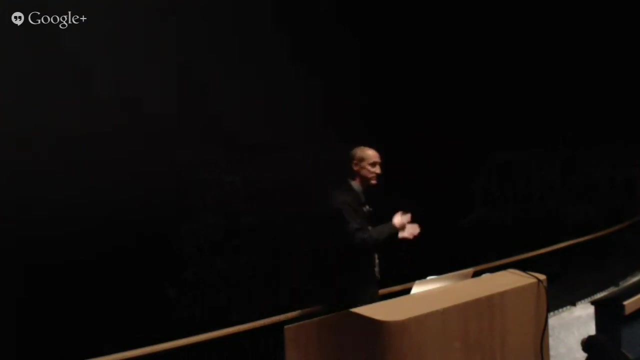 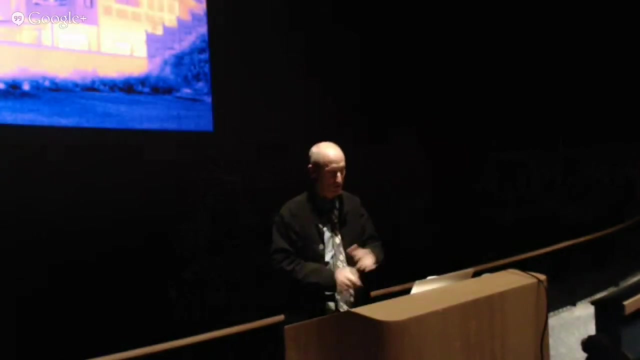 It's free. Good. So it may have come along with an infrared camera, So all day long it's sun's coming, it's out heating up the earth And your house. when it's making heat, they can take a picture with an infrared camera. 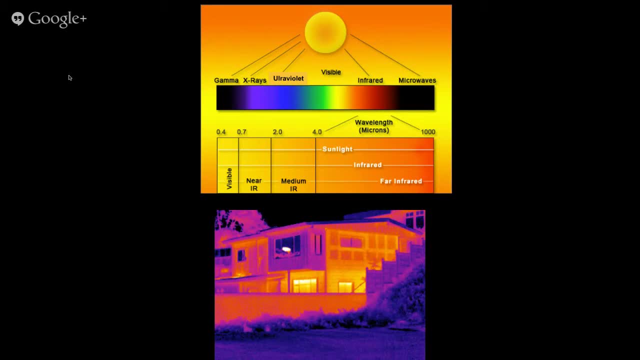 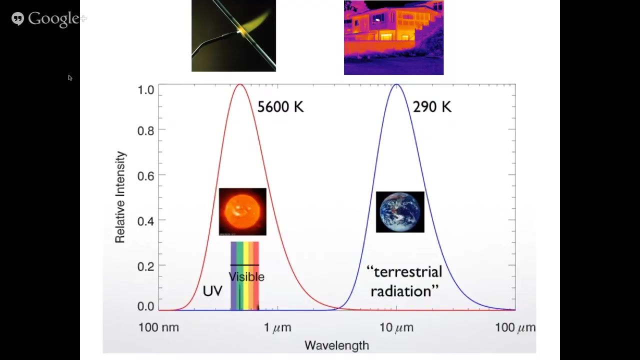 So you can't see that without a camera which is tuned to a certain part of the electromagnetic spectrum. And so the earth is doing that. The earth is receiving the radiation from the sun in the visible and it's emitting in the infrared. 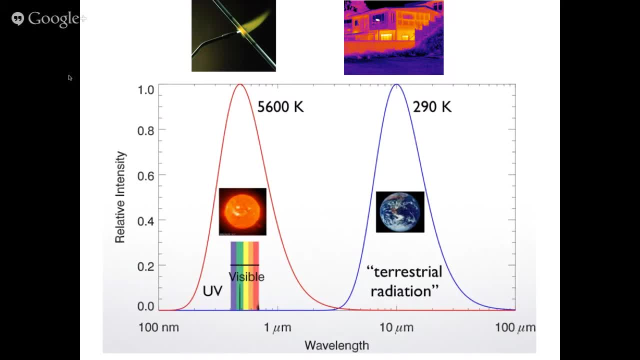 And you can see here this sort of cartoon- shows that there's a separation in the temperature associated with this part of the electromagnetic spectrum. So the earth's system really at its core, is driven by this process. We get visible radiation from the sun. 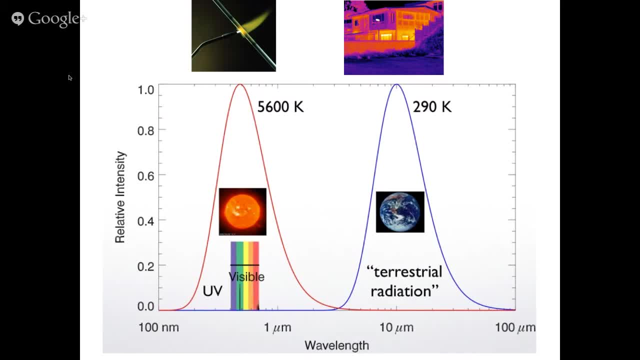 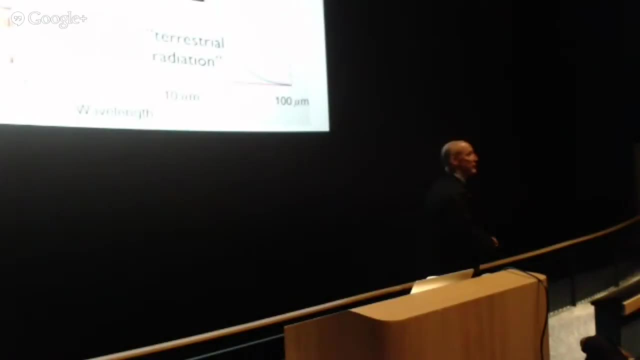 It heats up the planet as a system. The system is re-radiating, re-radiating this energy in the infrared. So how do these things balance? If you're not familiar with these things? radiation flows. You hear this, it's flowing. 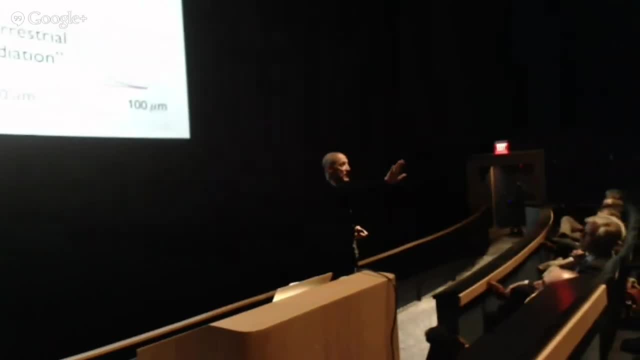 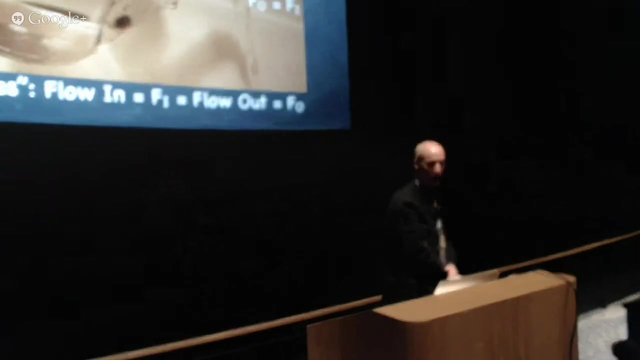 If you put your hand in front of a computer you feel something- thermal radiation. So it's just like the flow of liquid, So the flow of radiation. you can think of it in exactly the same way. I don't have much use for a grady boat like this anymore. 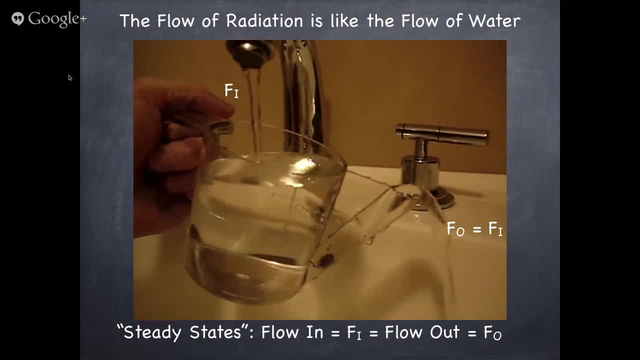 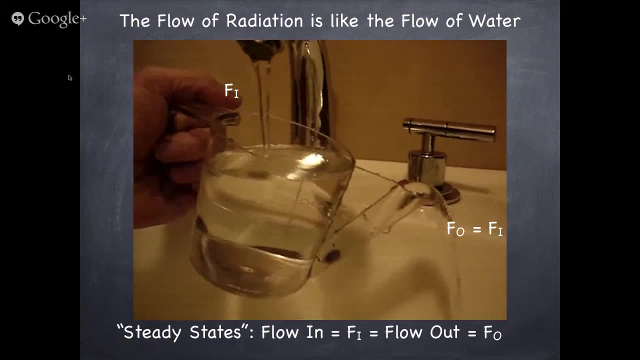 so I did this little experiment. You can see, we talk about what's called steady state. The flow in equals the flow out when the system's in steady state. You know that because the level doesn't change And you could have a different flow in and a different flow out. 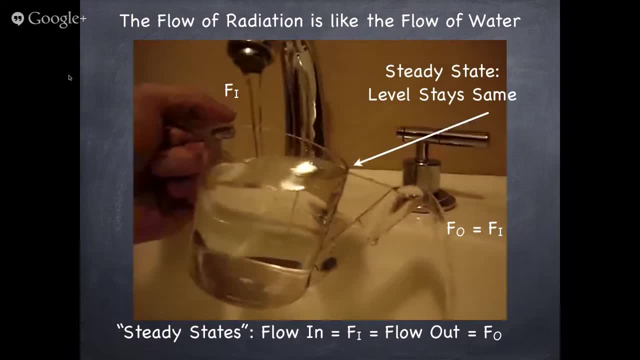 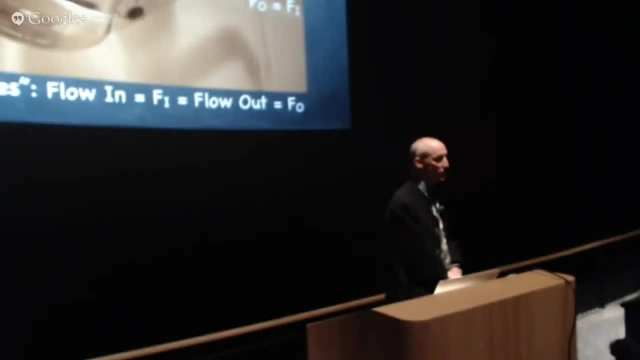 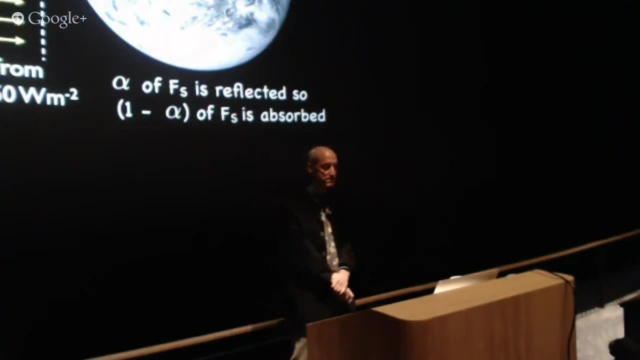 but they're the same, Then the level will never change So long as I can stand there and hold this. So you can think about the Earth system in a similar way, very crudely- that there's incoming radiation from the sun and a fraction is reflected by the planet. 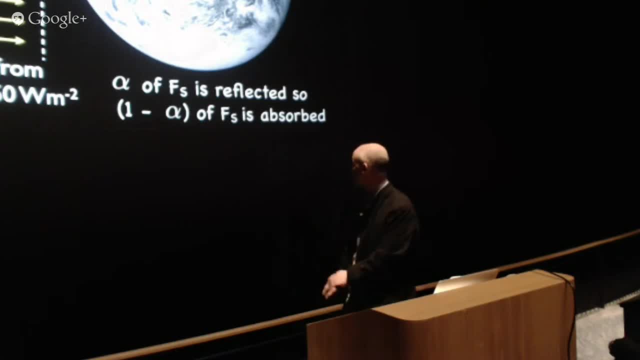 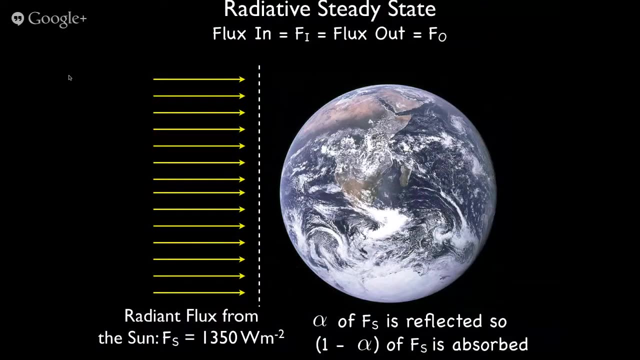 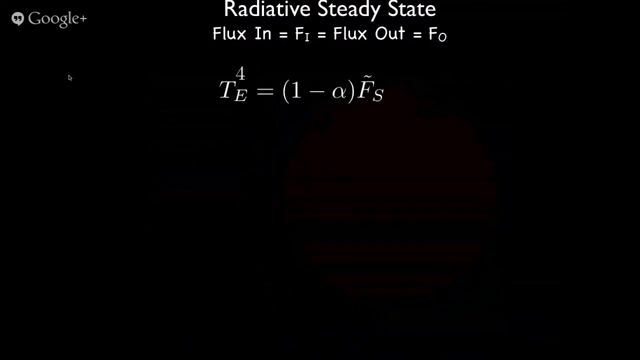 That's the albedo, which we call alpha. So a fraction is reflected and therefore one minus that fraction is absorbed. So we can balance those two things, treating the planet as a big rock, And when you do that you get the following instructive result: 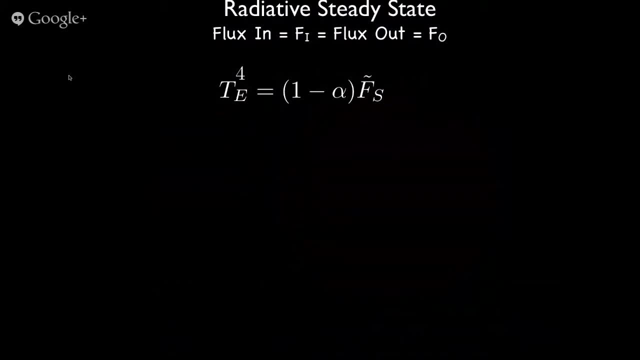 The fourth power of the temperature of the Earth is proportional to the solar constant times. this quantity here one minus the albedo. So if the Earth was, uh, completely white, the albedo would be approaching one, because all of the invisible radiation 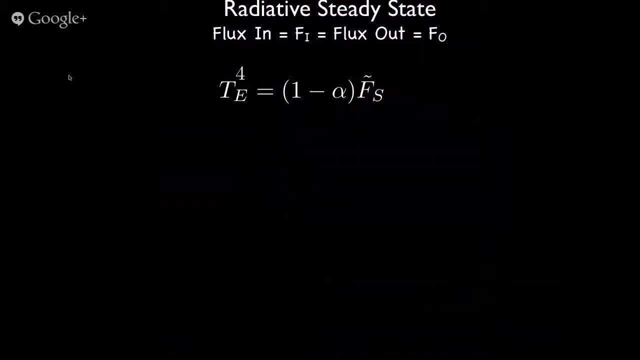 would be reflected. And so you can see clearly: as the albedo increases, one minus, the albedo increases and so the temperature of the planet increases. So the more white stuff you have covering the planet, the lower the temperature will be In this radiative balance. 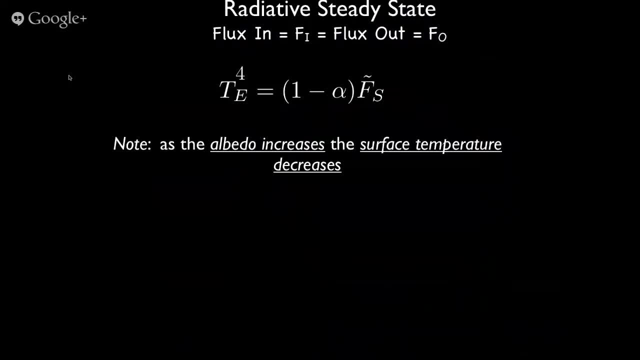 So that's the main message from such a simple argument. And if you just put in numbers for what we roughly estimated, the planetary albedo, then you get a temperature of about minus 15 Celsius or five degrees Fahrenheit, which is pretty cold. 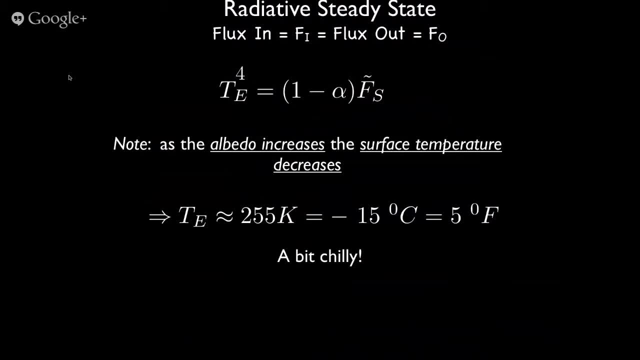 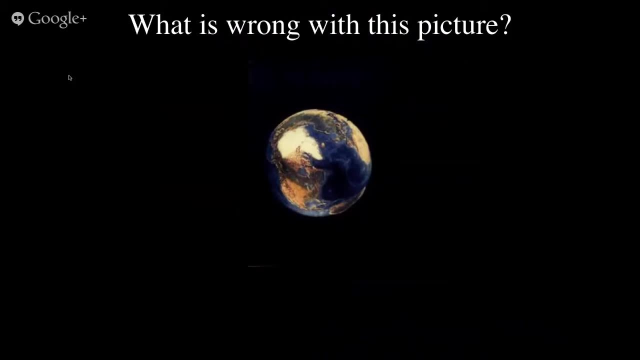 Even for Boston. But it's pretty close given the really crude estimate. I mean, it's not a thousand and it's not a milli-degree, It's pretty close. So what's wrong with the artist's rendition Clouds? 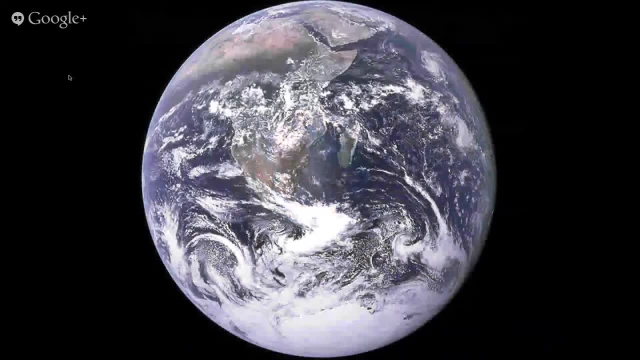 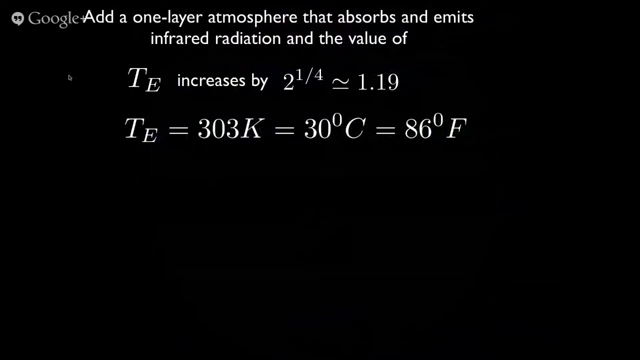 All right, so you know the atmosphere for a start. I mean we can quibble about the artist. Okay, so the atmosphere? So if we go through the same argument and just crudely put a layer of the atmosphere, 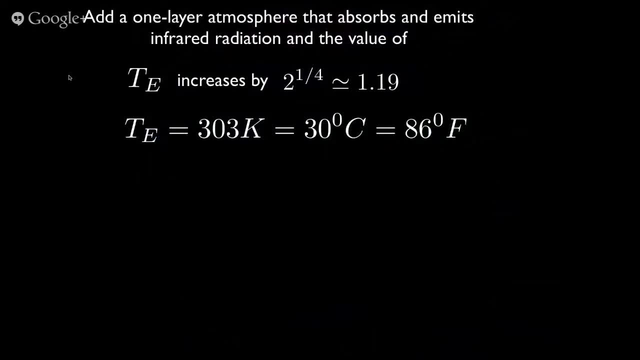 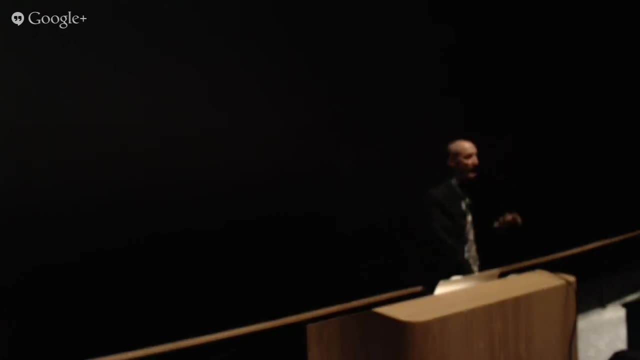 one layer of the atmosphere and that atmosphere is going to absorb the outgoing infrared radiation and re-emit some of it back and re-emit some of it back to space, And so you know, when it's a cloudy day here, it can be very warm. 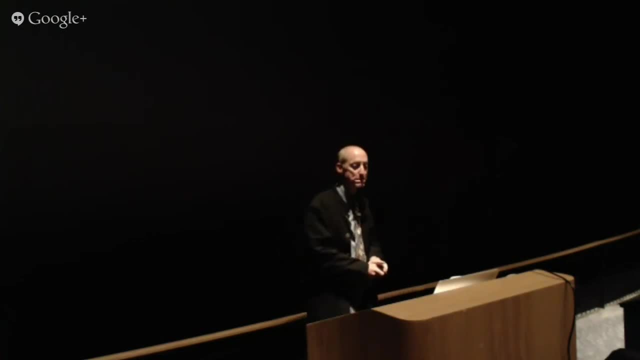 It can be very humid, It can be very cold. It can be very humid, It can be very hot, It can be very humid, It can be very cold, It can be very humid. So if you just do that exercise, you find that the temperature. 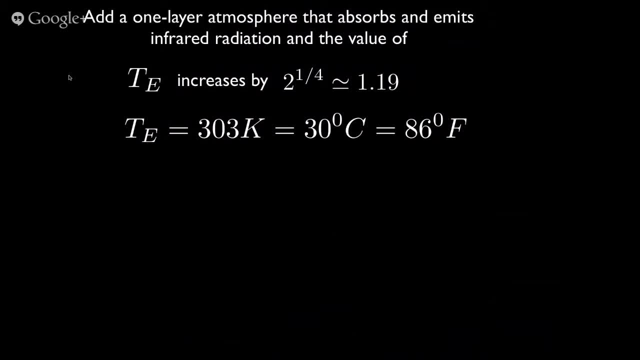 of the surface increases by about 1.2, relative to the previous number, And so then one gets the value of about 86 degrees Fahrenheit, which is of course pretty warm too. But you see the qualitative trend, And of course, 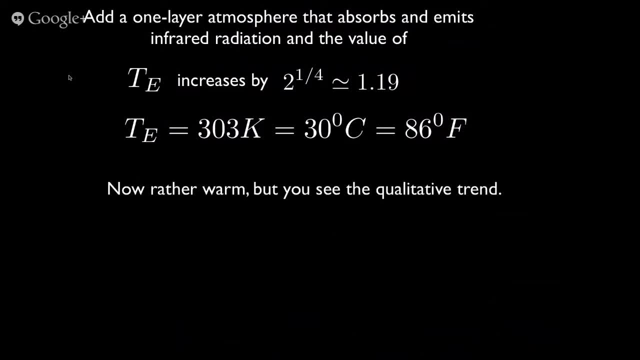 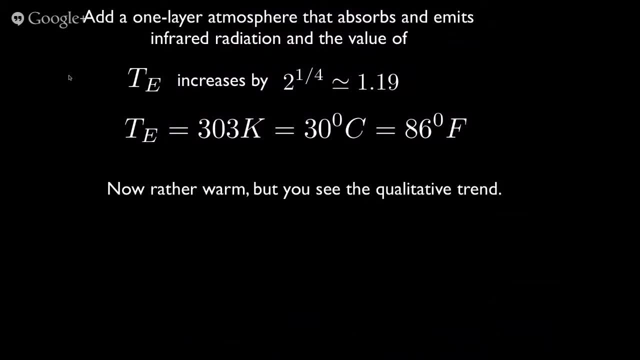 And what scientists would do is start putting in more layers and start putting in more complexity and trying to figure out you know what controls the temperature of the surface of the Earth. But my point here really is that the albedo is a very important quantity. 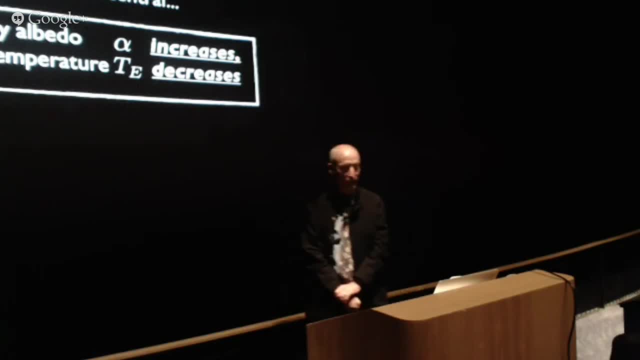 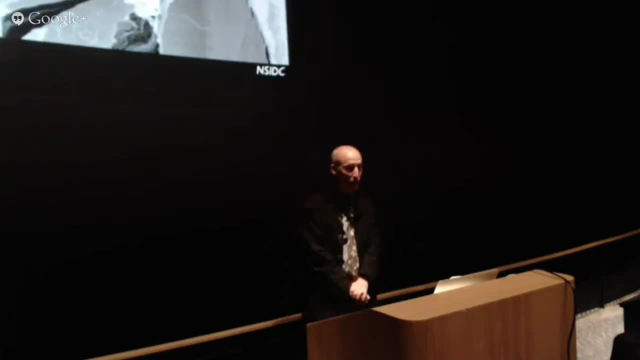 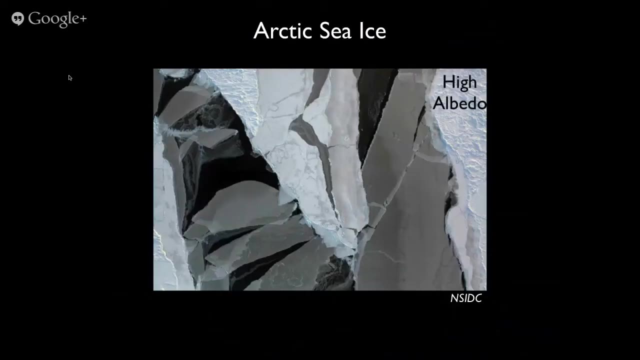 in that the albedo if it increases, the planetary temperature decreases And when we look in the polar regions, we can see that this vernier of ice really playing an interesting role in that regard. You have regions that are very reflective, with high albedo. 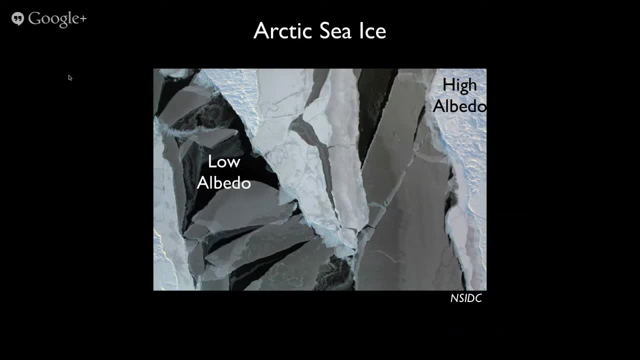 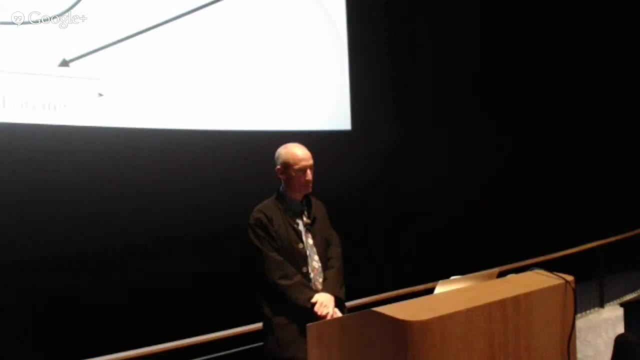 And you have the open ocean, which absorbs a great deal of radiation. So the albedo of the ocean is about 0.2, and the albedo of this ice is about 0.65.. Okay, so this is a very interesting. 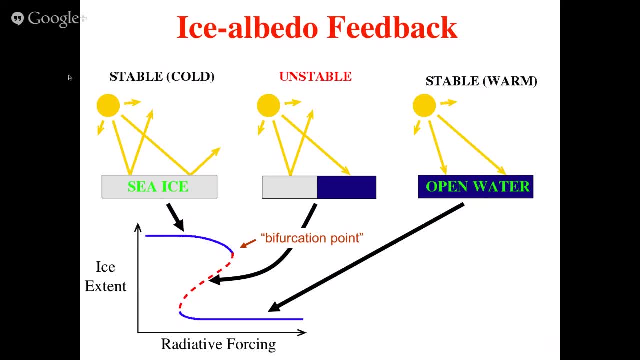 idea. This idea is invoked in what is called the ice albedo feedback. So you can imagine- you know I've just drawn a cartoon with the ice extent over there and an increased value of radiative forcing. you can imagine when you turn the sun. 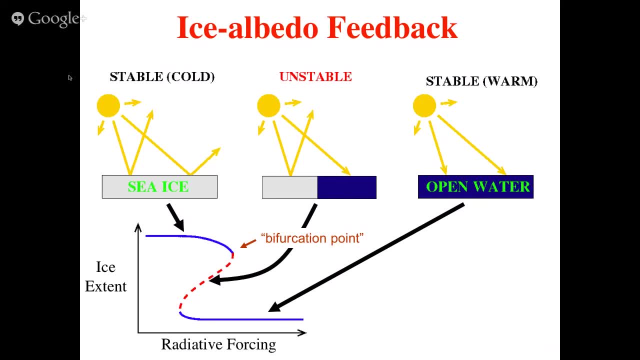 for example, And the blue curve is the case where you have a lot of ice, like we have today, and there's a lot of radiation being reflected- And the blue curve is the case where you have a lot of ice, like we have today. 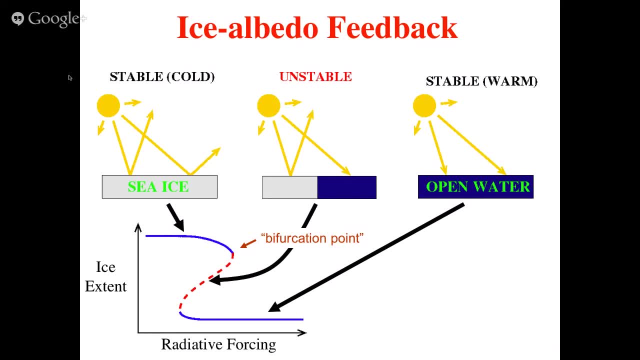 and there's a lot of ice. Now you can imagine warming the system and increasing the aerial fraction of water relative to ice. That will allow more radiation to be absorbed into the system, which will heat up the water, which will melt the ice. 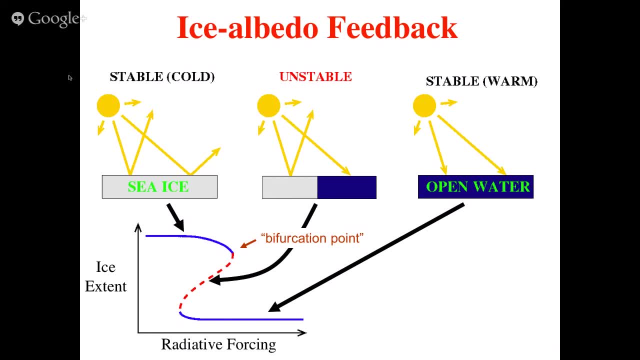 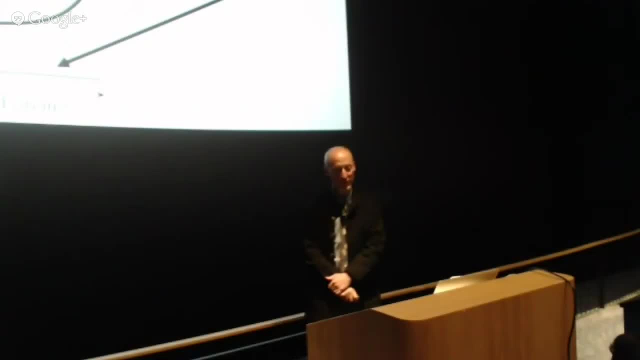 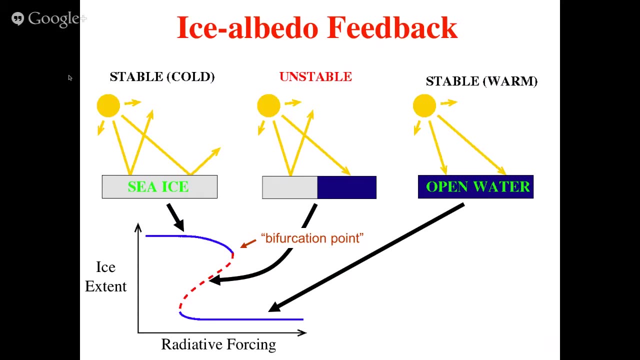 And eventually one can theorize that there's a threshold beyond which the ice experience will drop from this value up here on the left to a low value. We call that a bifurcation point. It's really something that people worry about. 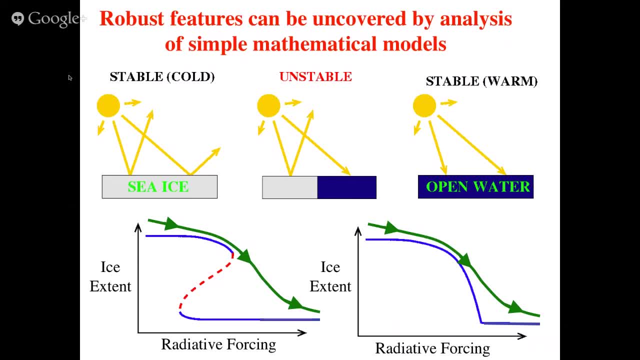 Now, practically speaking, whether the curve looks like the one on the left or the one on the right is probably not an issue for humankind per se, but it's a scientific issue for us to understand what's the nature of the ice in the Arctic. 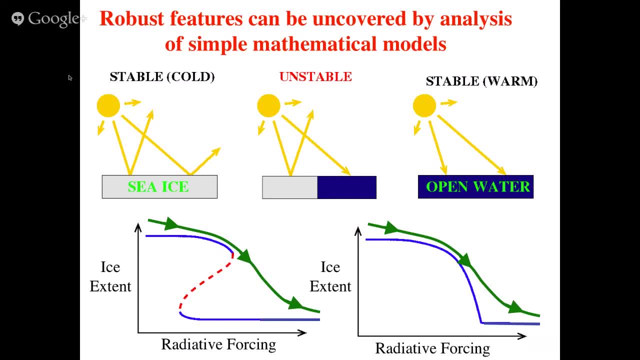 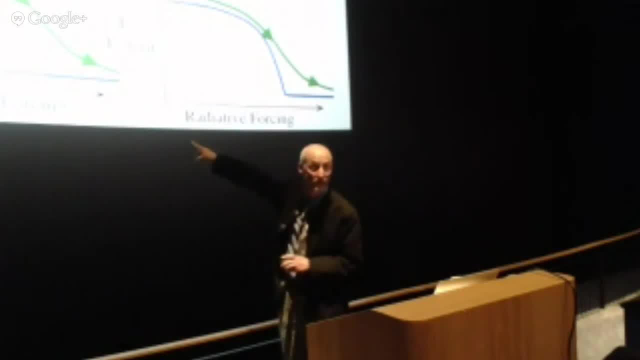 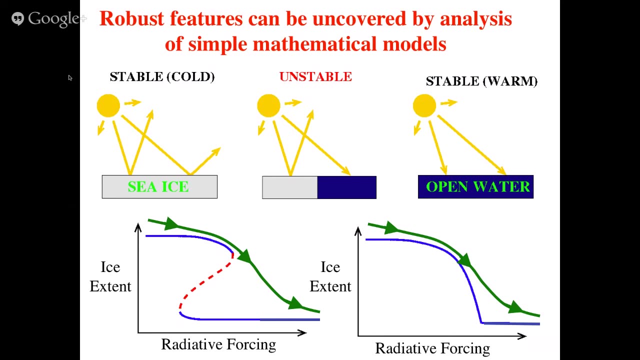 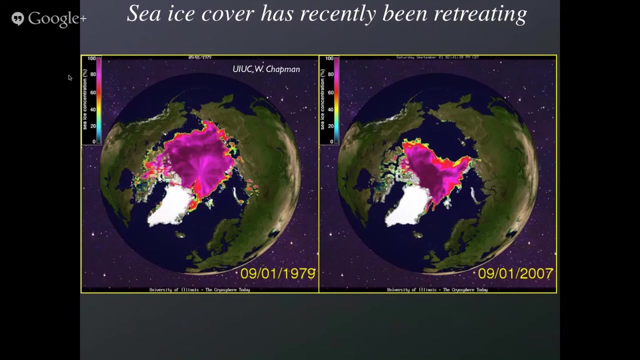 So if you reduce the weight of the force thing, you just increase the ice extent, Whereas this one requires you to go all the way back to where the dotted red line hits the lower blue line and then jump up So you can. 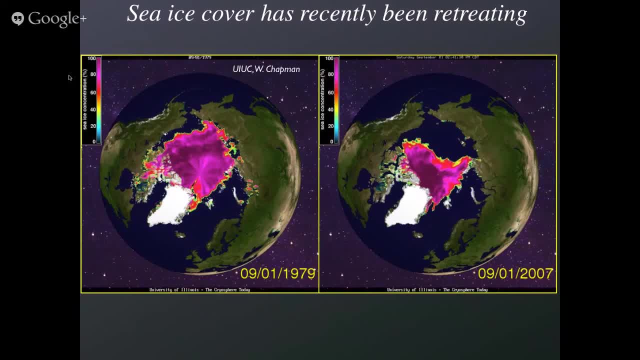 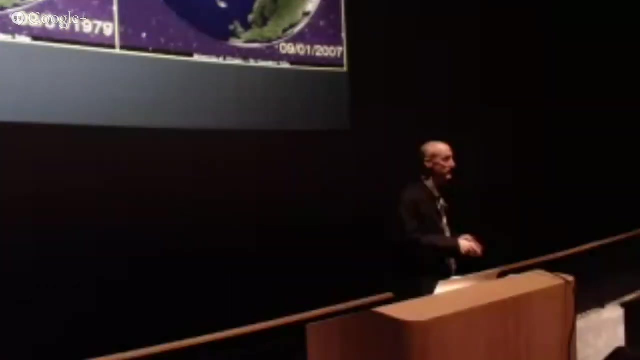 see those and you read about it all the time because reporters have to say something's happening. But this is why You can go to this website, which is Cryosphere. Today, Bill Chapman has been archiving this data and you can go and look. 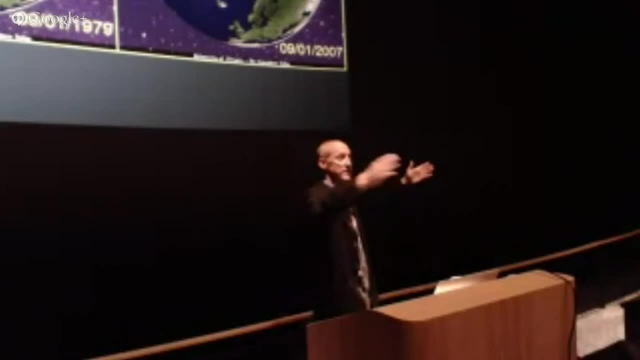 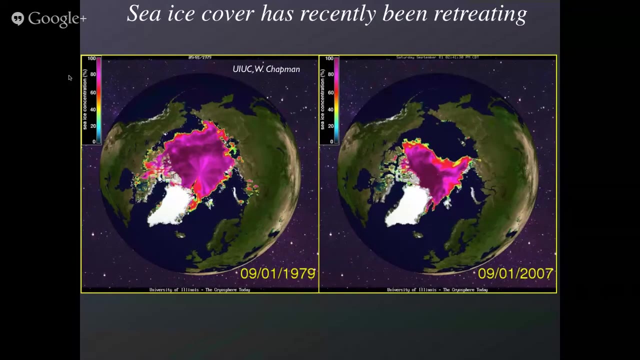 at any day. look at your data, look at what's going on in the world. So you can go and look at your data and look at what's going on in the world, So you can go and look at this transition that people 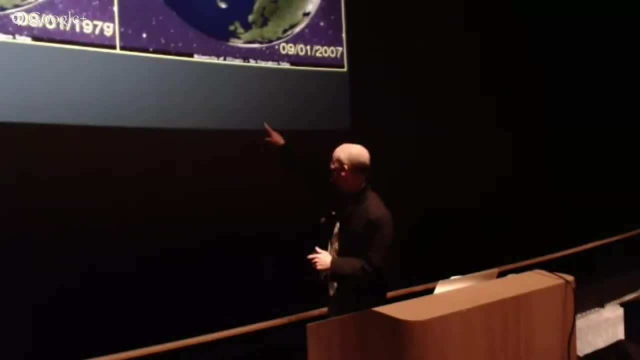 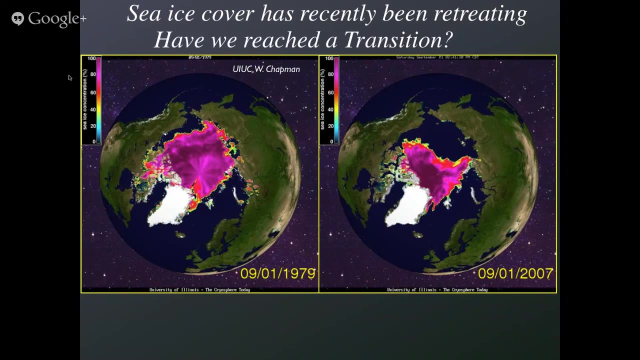 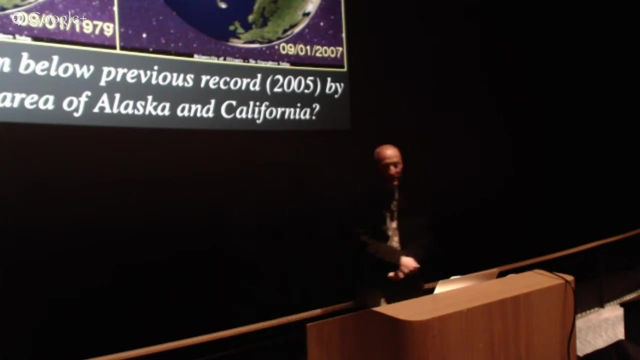 are focused on Now. you see here the dates are in the lower part. This is the first September of the satellite era and this minimum here in September of 2007. many people say, well, there's some transition relative to the previous year, which is 2005. 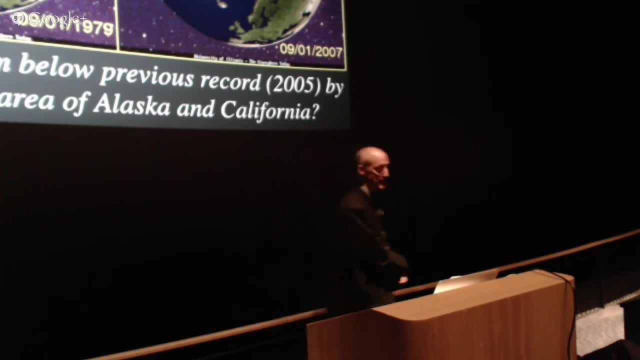 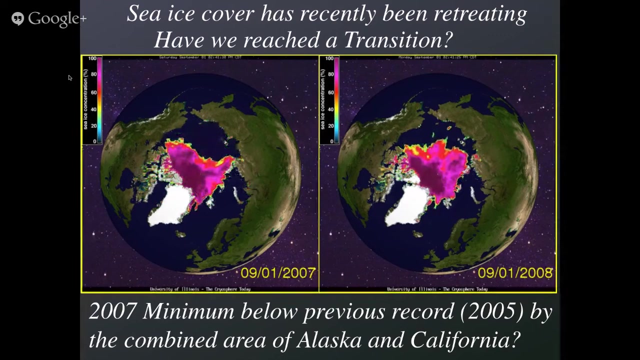 by about the area of Alaska plus California. There's a major change in the area extent of the ice, So now I'll flip to moving September 2007 to the left and we'll just go back to 2010,. 11,. 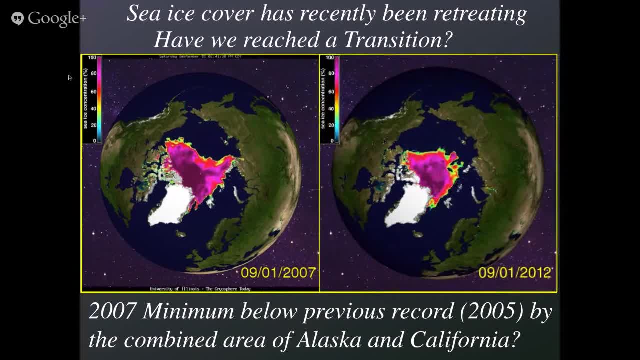 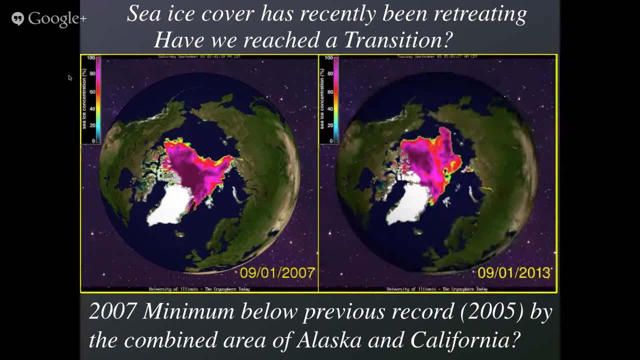 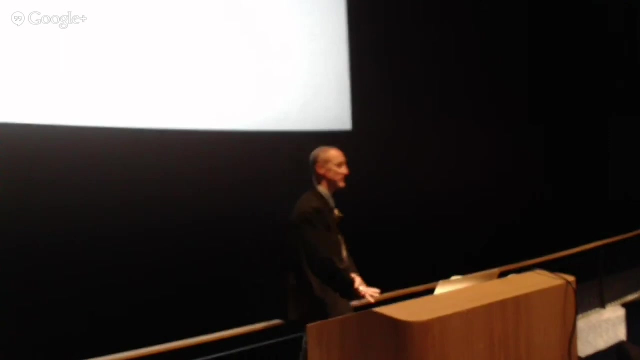 12,. that one got a lot of press, and then just last year. So you might say: well, what does this have to do with the press of 15?? I don't know. I think it's a little bit more complicated than the. 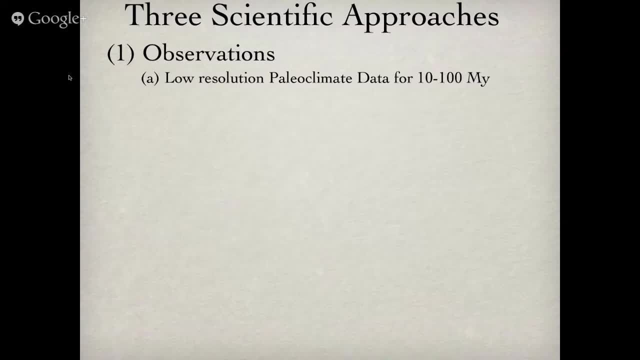 previous year, But I think it's a little bit more complicated than the last year. So I think that that is a little bit more complicated than the last year. So I think it's a little bit more complicated than the last year. 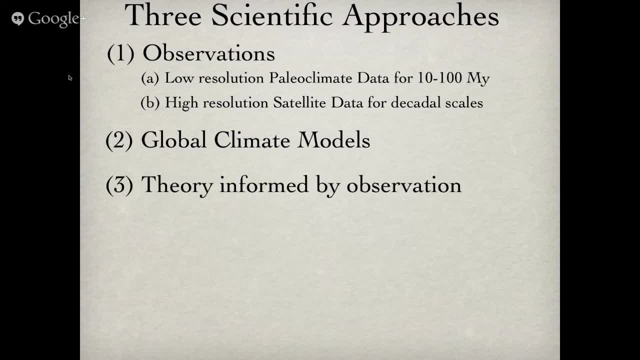 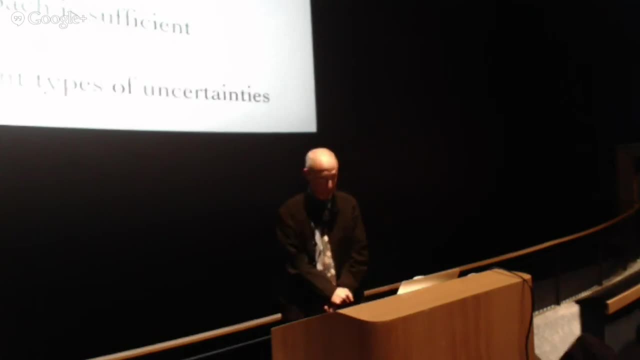 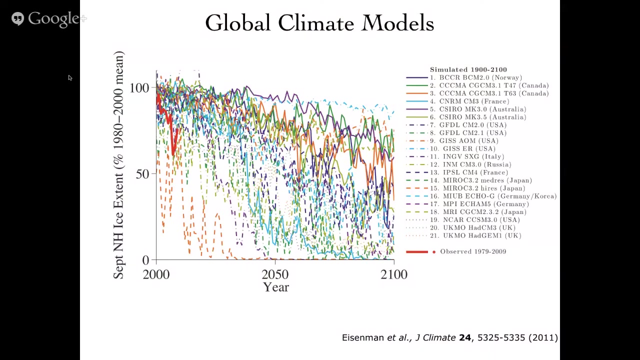 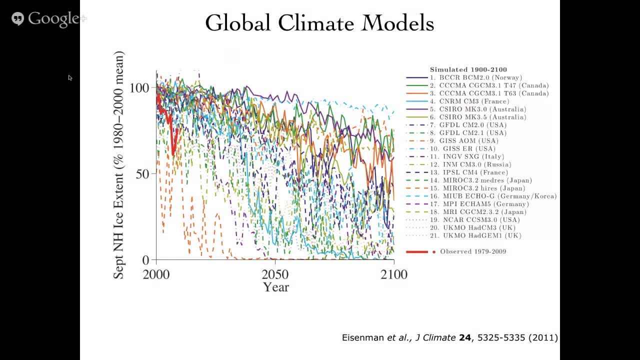 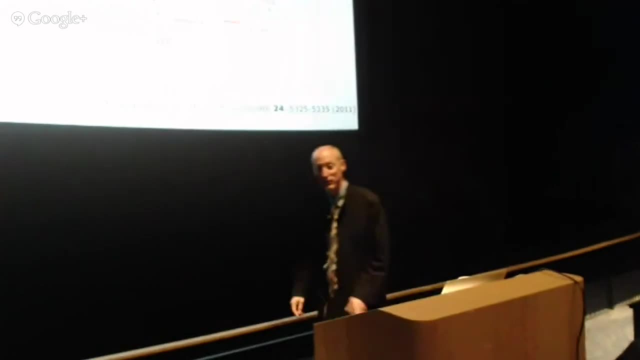 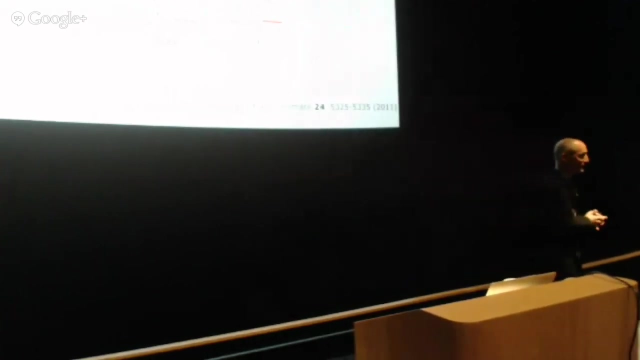 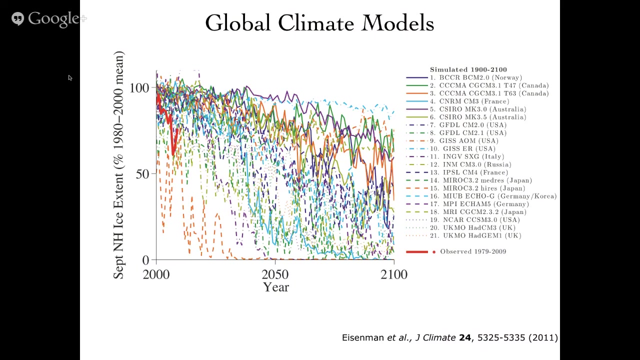 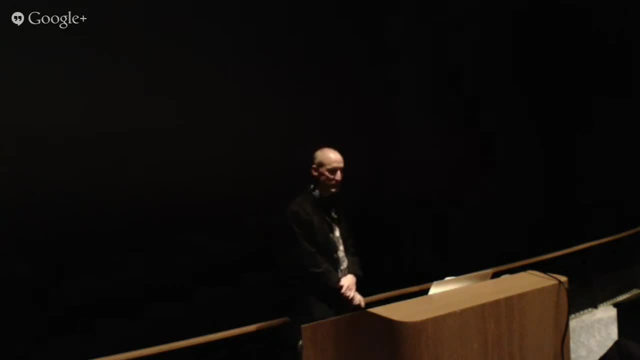 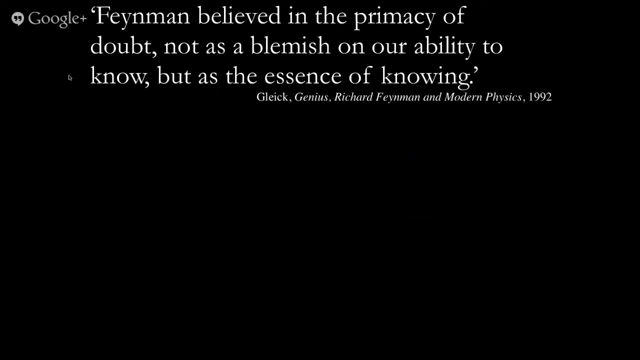 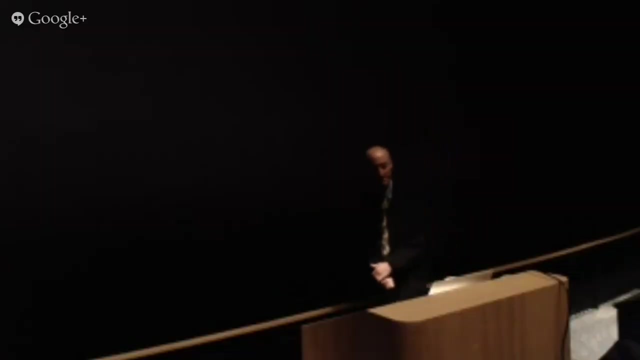 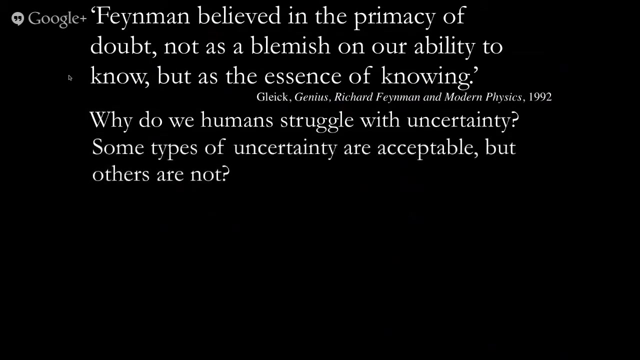 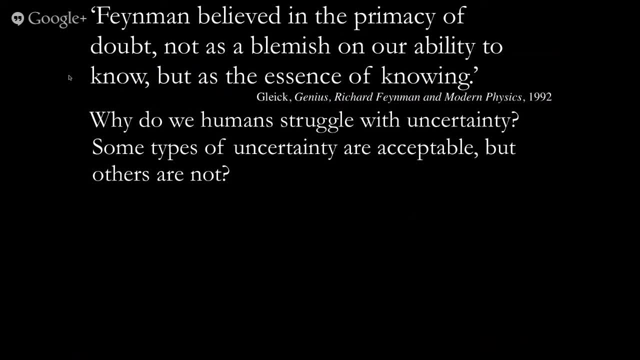 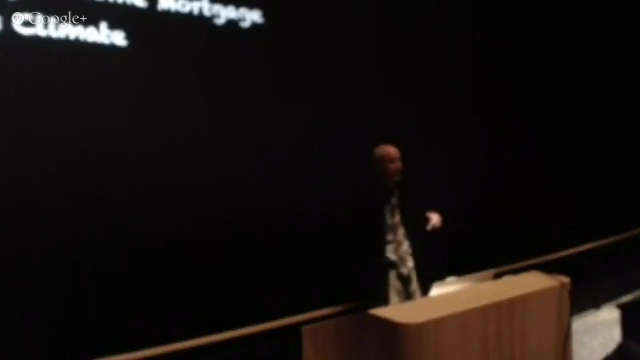 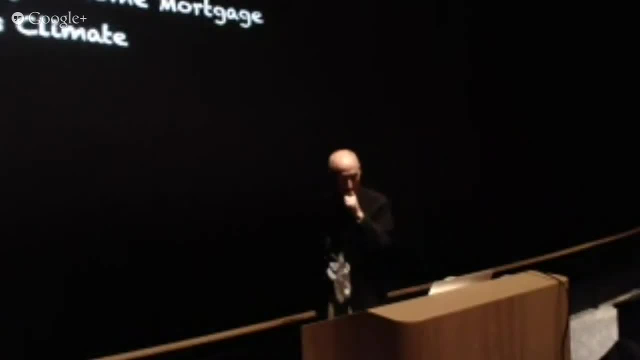 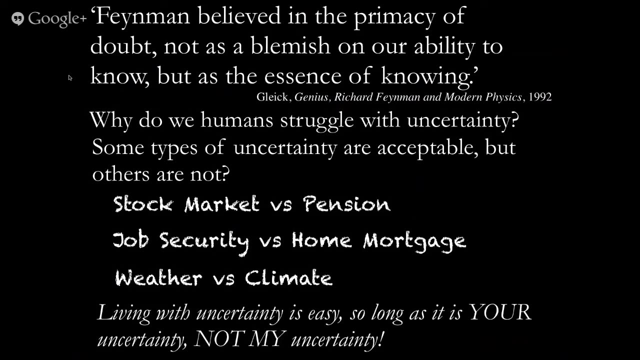 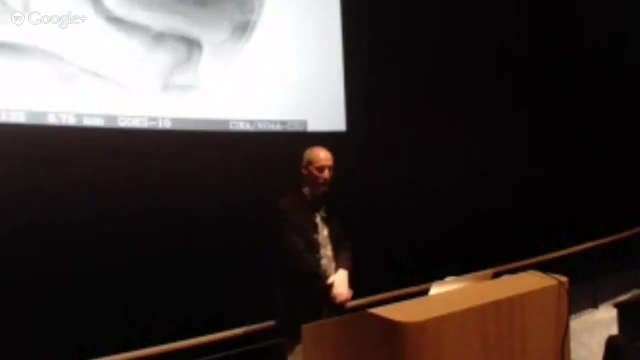 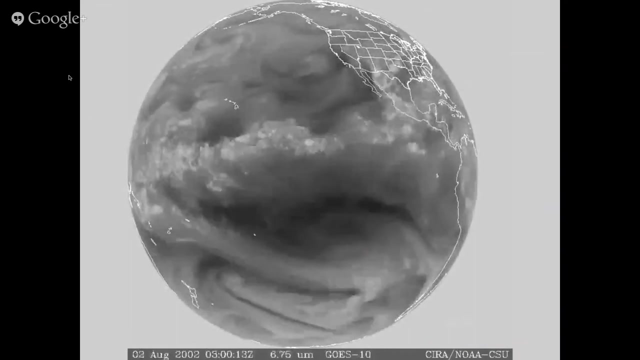 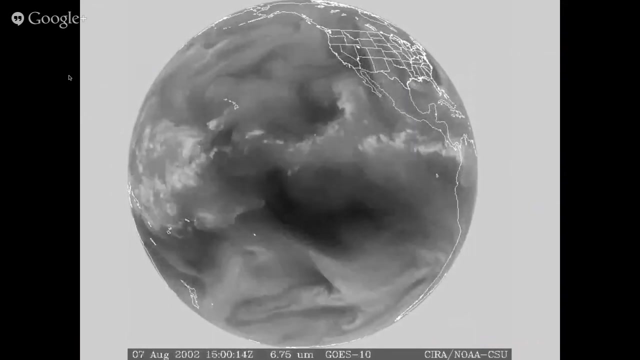 the last year, So I think it's a little bit more complicated than the last year. So let's start to peel back those things here. Here's a picture of the atmosphere at about 10 kilometers. the moisture in the atmosphere. 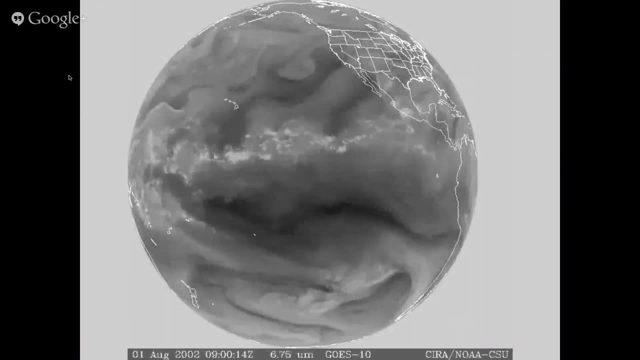 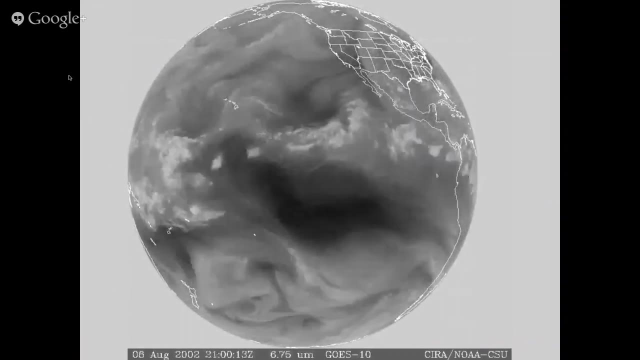 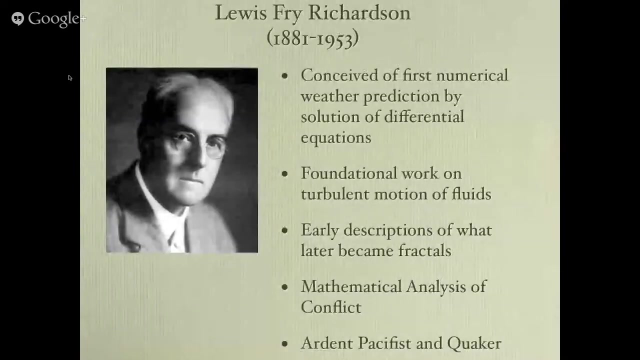 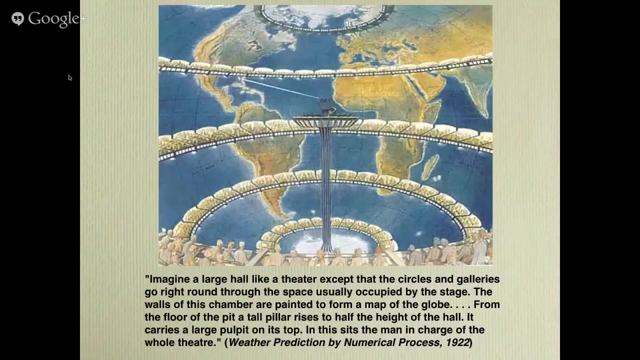 This is a really beautiful movie. You can see that there's a lot of water in the atmosphere. So you can see that there's a lot of water in the atmosphere. So you can see that there's a lot of water in the. 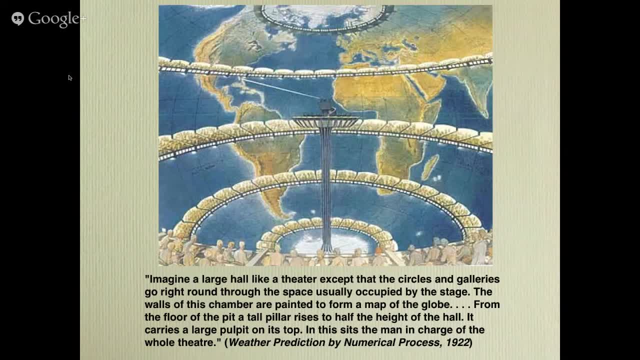 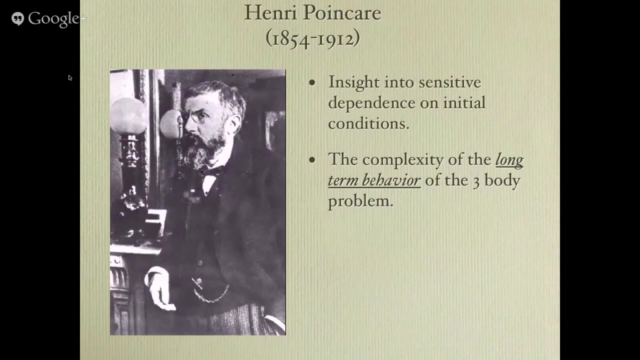 atmosphere. You can see that there's a lot of water in the atmosphere. You can see that there's a lot of water in the atmosphere. So you can see that there's a lot of water in the atmosphere. So you can see. 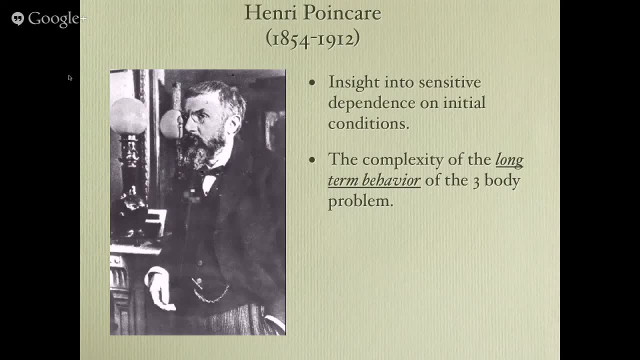 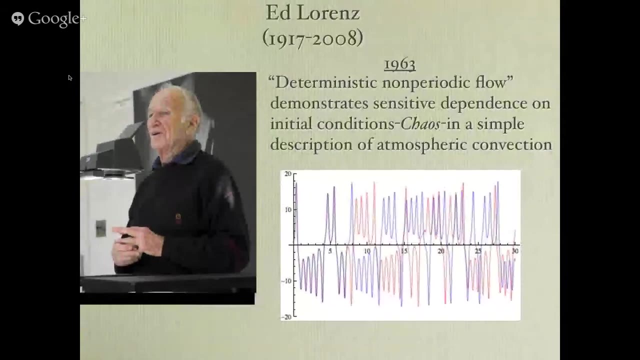 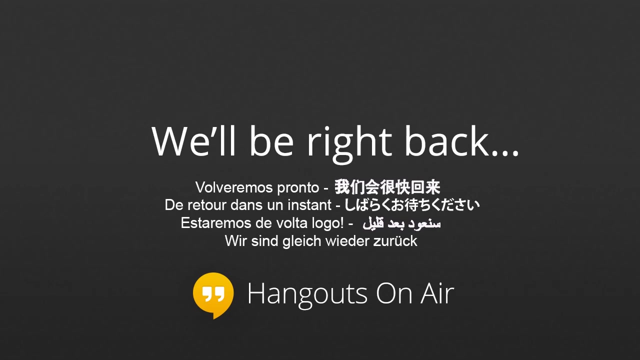 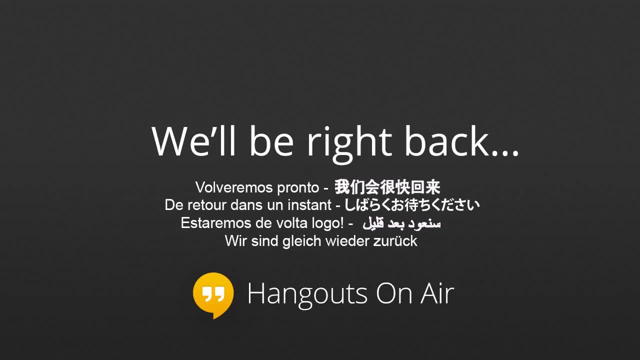 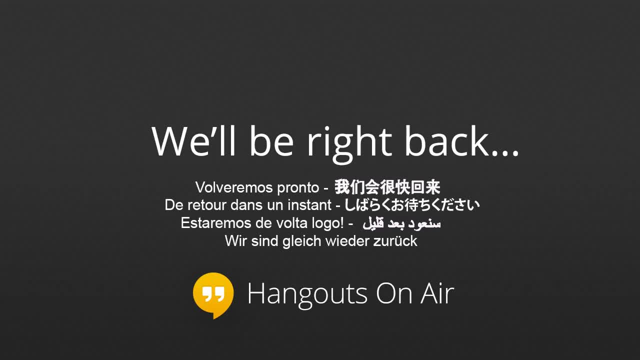 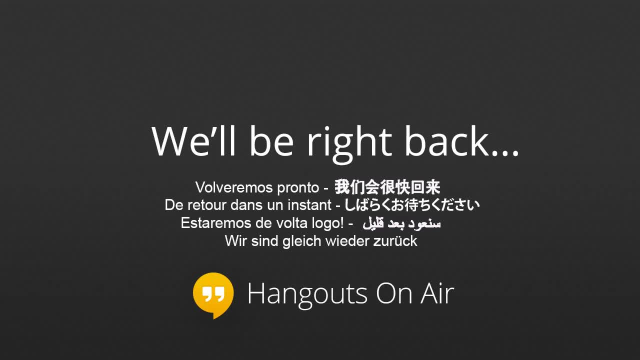 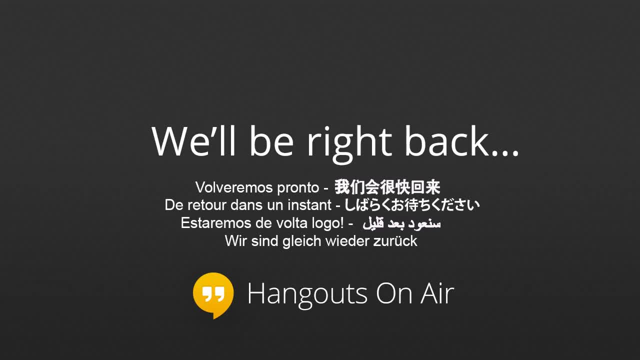 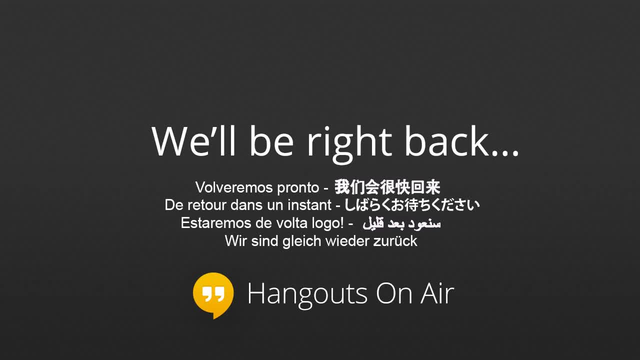